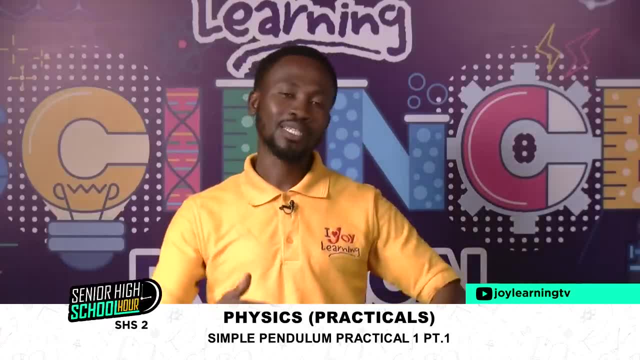 Usually people will say the question has got two parts: The practical aspect and then the part b- the question- The practical aspect- and then the part b- the question- The practical aspect- and then the part b- the question- The practical aspect- and then the part b. that will asks you short questions about the. 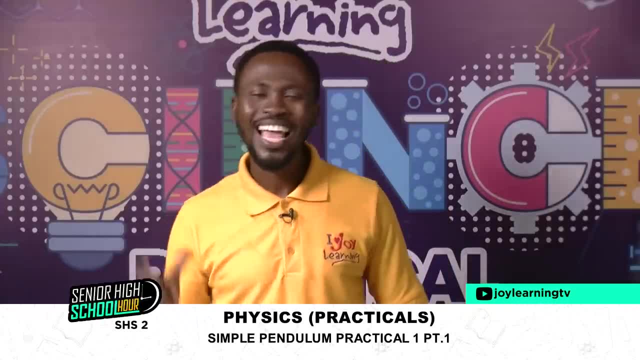 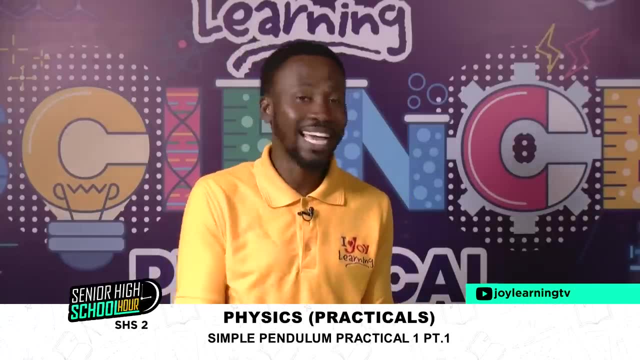 practical. But I'm saying it has got three parts, why Every question starts with a diagram And you have to look at the diagram. I call it to look and do So. you look at the diagram, the setup is there, which we call the experimental set up. 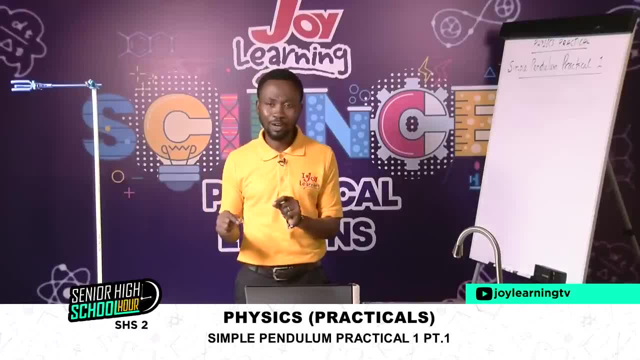 It's a diagram. Then you look at the diagram, watch what's in the diagram and try to also do a similar thing. Right? So I have a diagram, Watch what's in the diagram. You have A. What is different I am using? 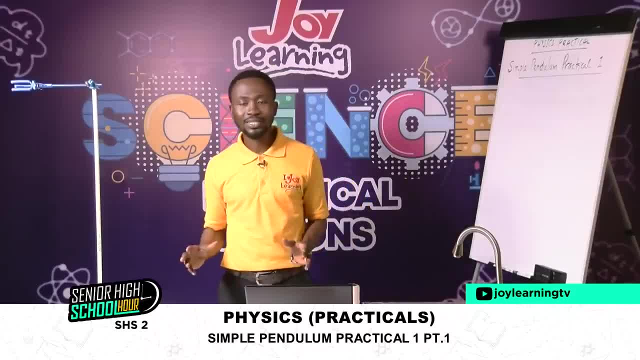 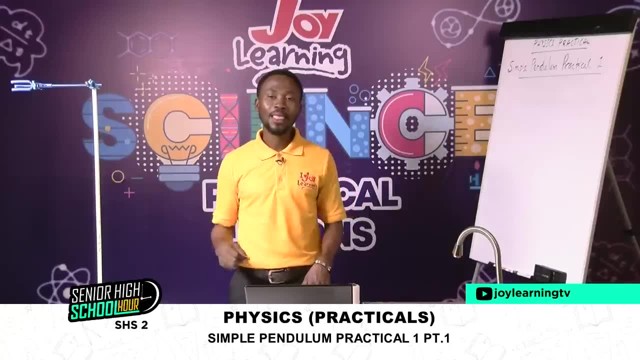 Hello, everyone say hello. Tapi lovea la property is understanding what we have here today. here in my diagram, I can see a rater stand on a bench, I can see a clamp, I can see a thread and I can see a pendulum bulb. now, after that, the experiment will. 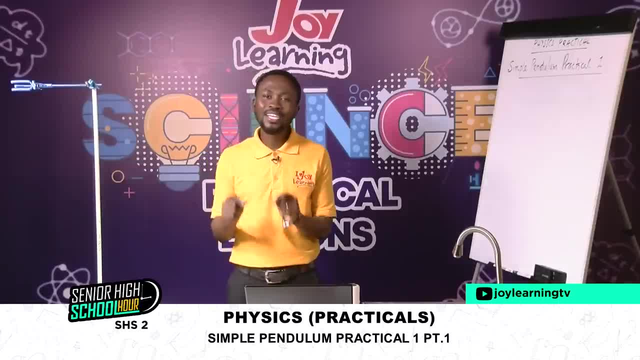 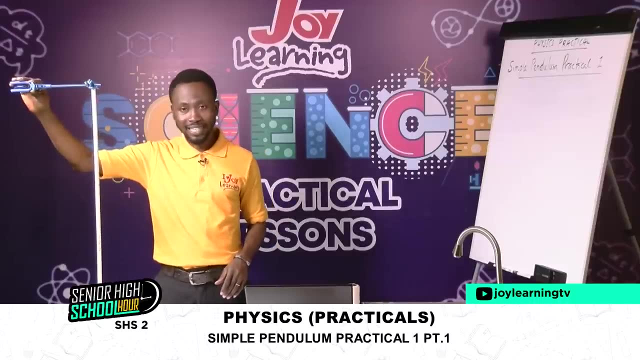 give you what you call the apparatus so you make sure that everything stated in apparatus is available to you for the experiment. in my apparatus I have what you call a rater stand. so this is what you call a rater stand and that has a clamp attached. 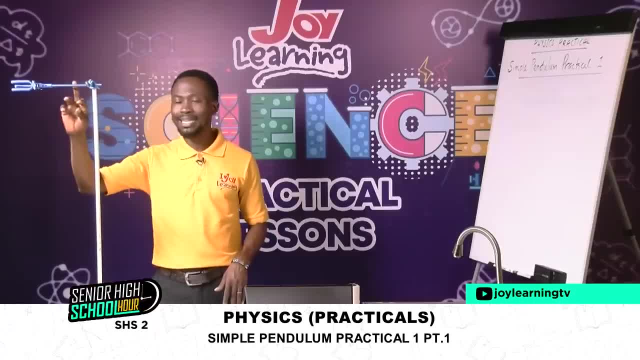 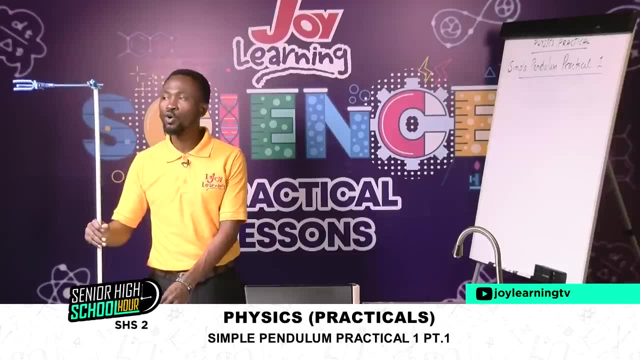 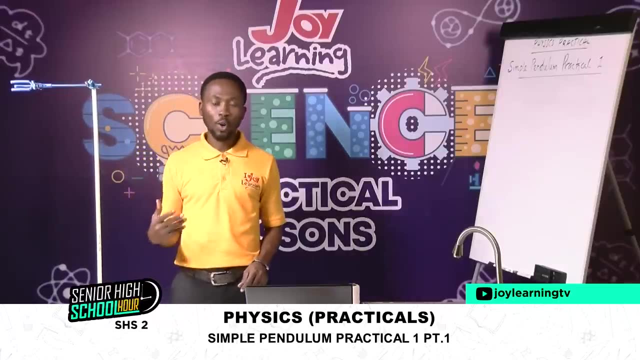 to it. so that's a rater stand and then a clamp. make sure that your rater stand is on a flat surface and it shouldn't be shaking as you go through the experiment. if it shakes, then there's a problem. then I also have what you call pendulum bulb. this is 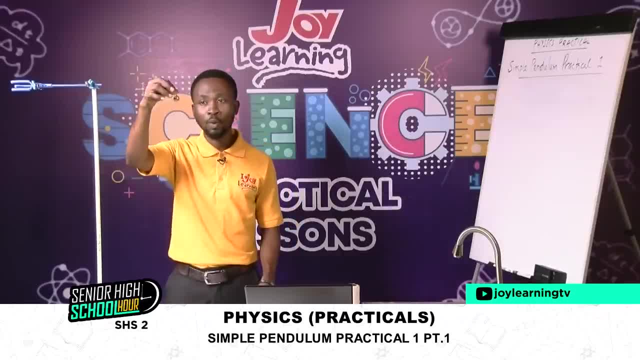 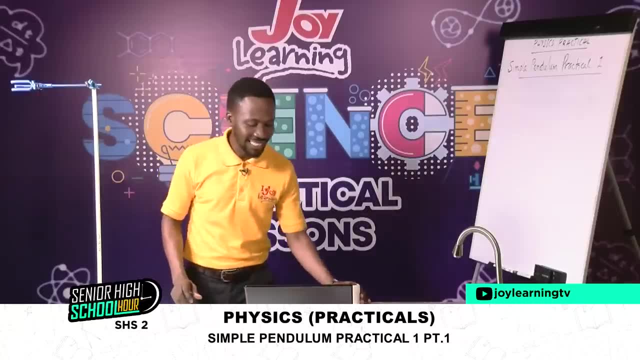 what you call a pendulum bulb- b-o-b. a pendulum bulb. that is it. so I'm going to add a pendulum bulb b-o-b. a pendulum bulb. that is it. so I'm going to add another thing, a string to it. then I have in extensible thread- and this is my in- 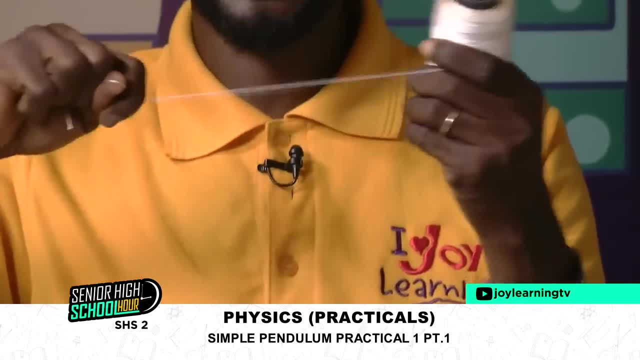 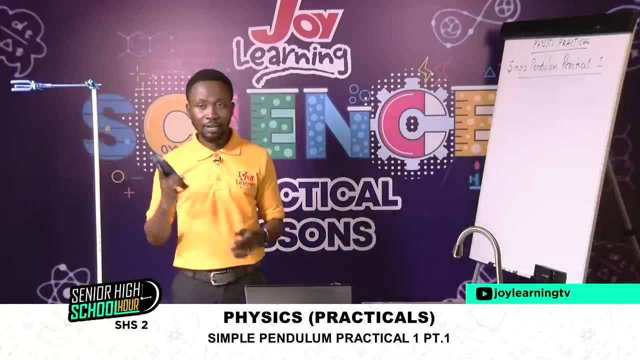 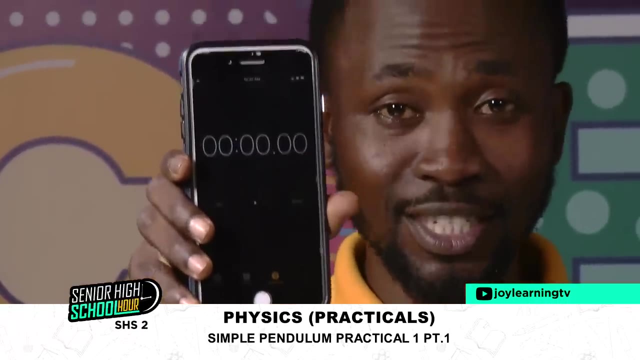 extensible thread. it shouldn't stretch, it shouldn't be an elastic material. no, that is it, then, a stopwatch. so I'm going to use a stopwatch for my phone. that is my stopwatch. you can see, on a stopwatch, you can see zero, zero, zero, zero, zero, zero. 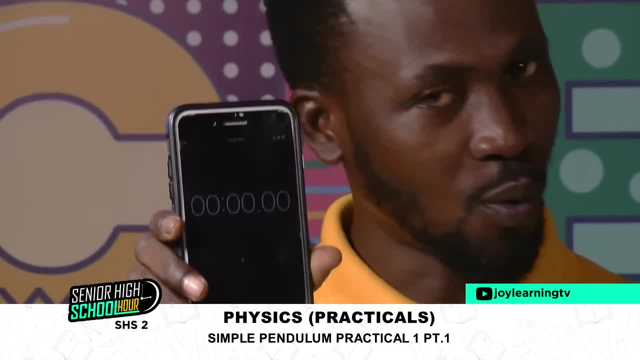 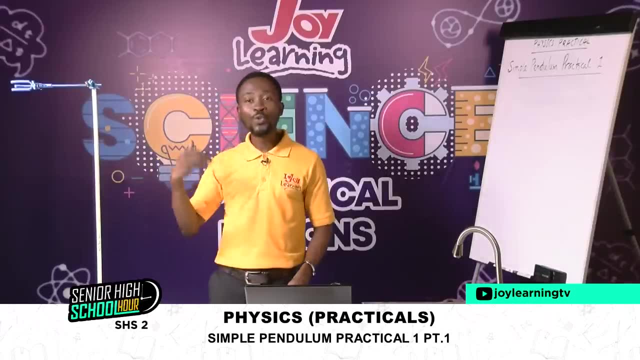 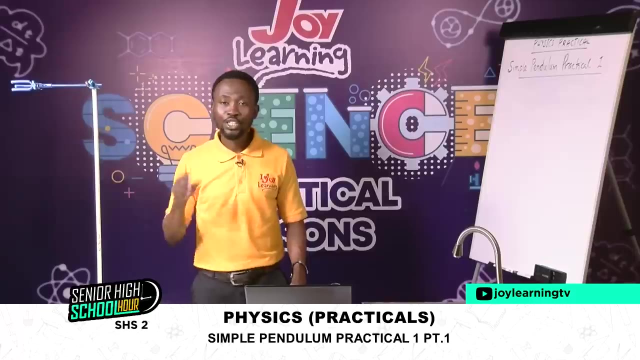 I want to show you how to read from the stopwatch. good then, we are good to go. the next thing I'm supposed to look at is you try and you read the question from the first word to the last word and make sure that you understand the question. that is very critical and that is very important. if 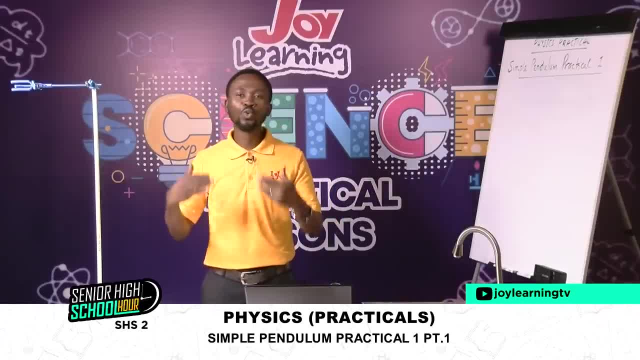 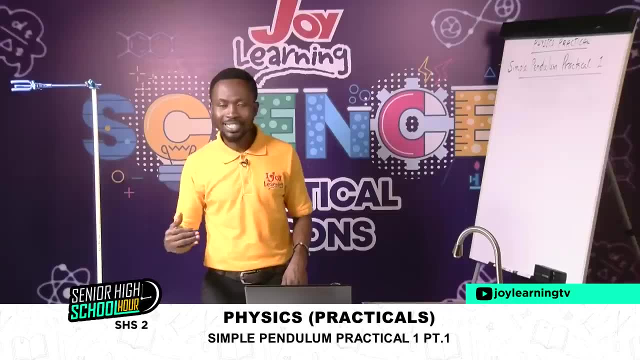 you don't make a head and tail out of the question, you won't be able to carry out the experiment successfully. so you have to read the questions, try to figure out in your mind what the question is about, and then you try to do all your acts to do so. 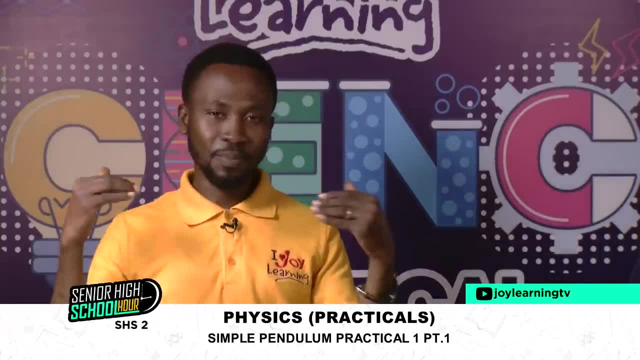 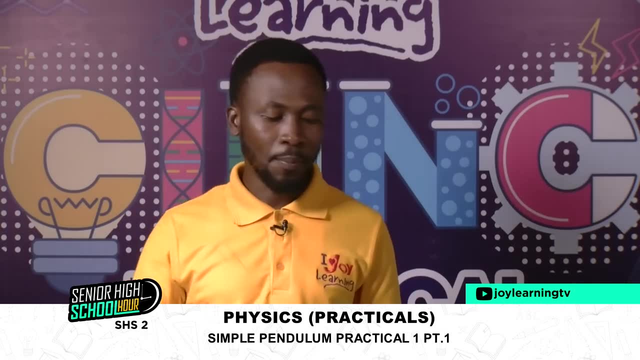 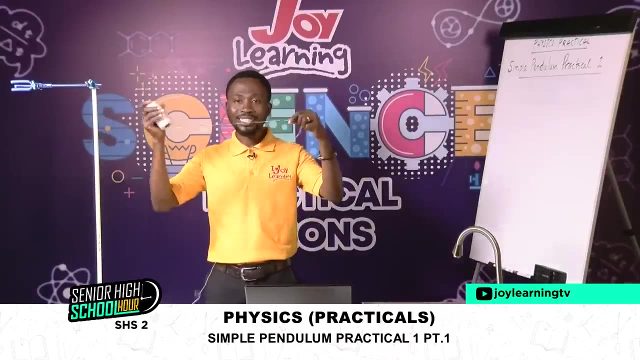 I'm going to take time and read the question, explain the salient points, and then we look at what to do. we are told that you are provided with a pendulum bulb and a 120 cm long thread, so it would be better for me to start with measuring the length of my in extensible thread. 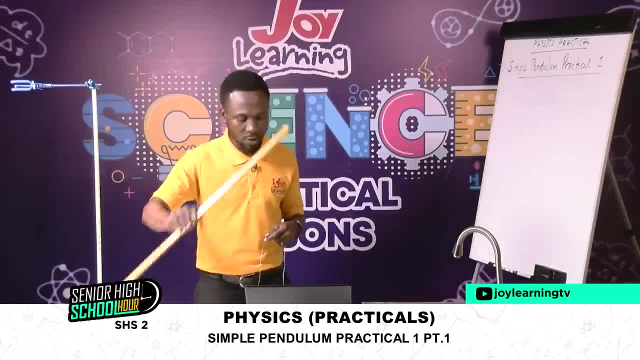 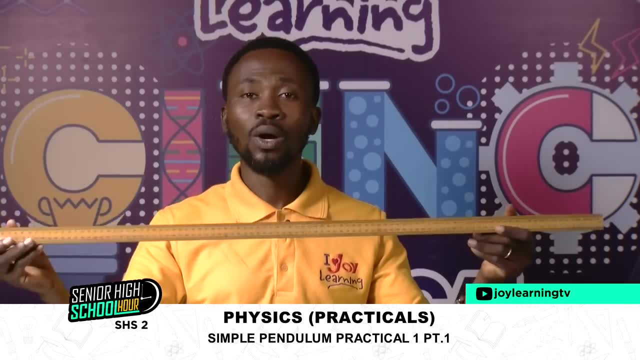 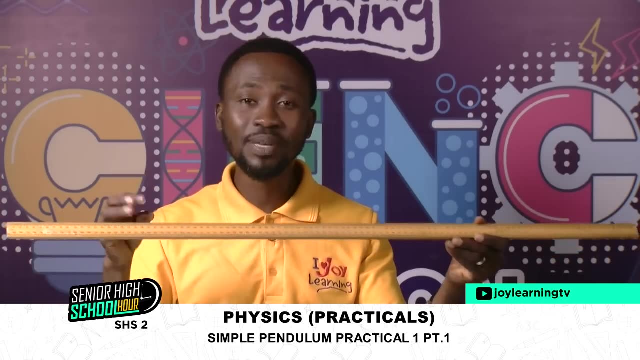 so I pick my thread, then I pick my meter rule. I also need a meter rule. it's an apparatus, so that's a meter rule there. a meter rule is a rule that is 100 cm long, which is the same as one meter. the calibration is in centimeters. so although we call it a meter rule, 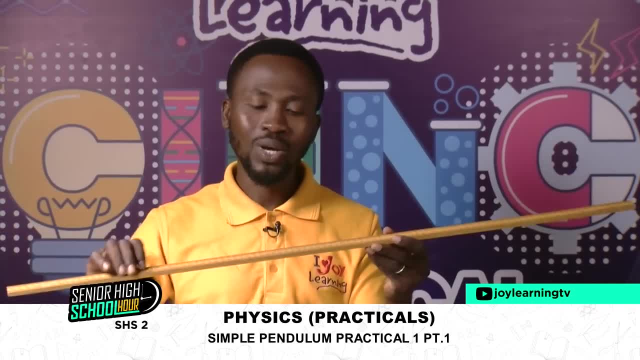 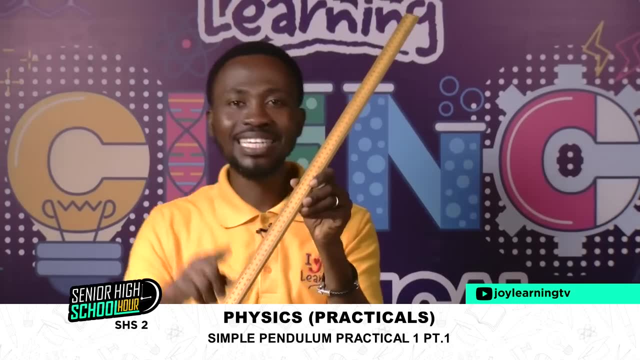 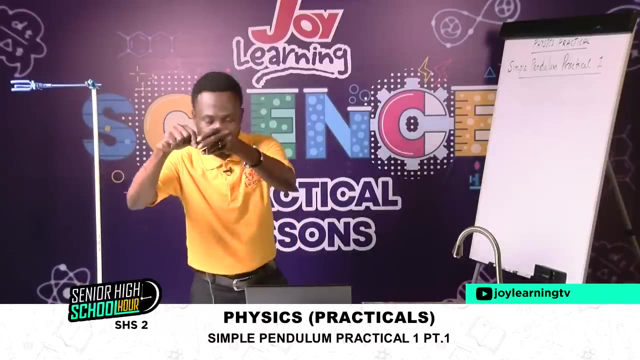 it is a 100 centimeter rule, so any reading you take from the meter rule should be in centimeters. the calibration has been done in centimeters. good, so I'm going to do the measurements. I'll pick one end of my thread, take it to one end of the rule, stretch it to the other end and that. 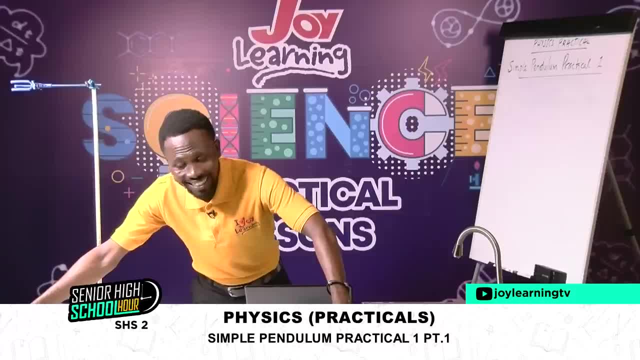 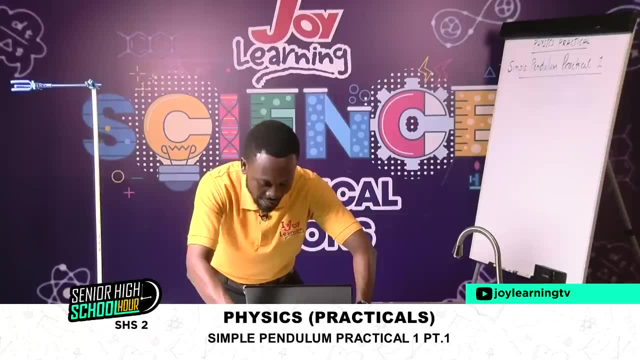 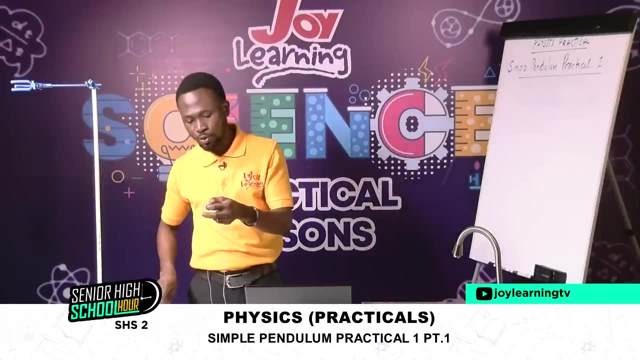 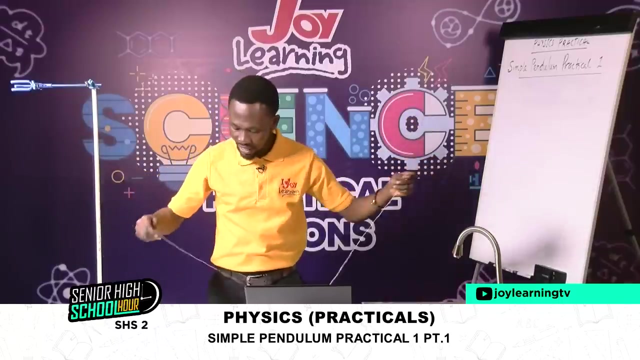 gives me 100 centimeters, that's 100. then now I'm going to add an additional 10, 20 to it. so from one end to 20, that is it. so where my 20 ends, I'll hold that place firmly. then I will be able to freely get that done. your alarm assistant will help you to cut the thread. 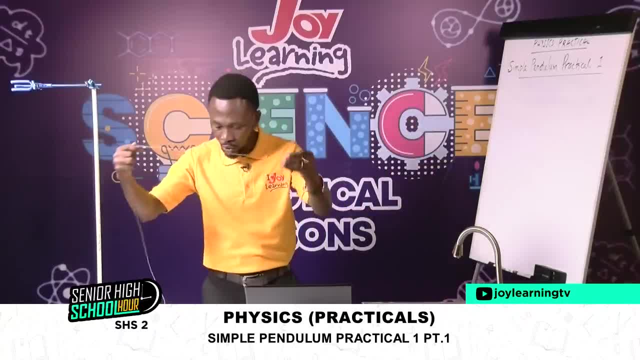 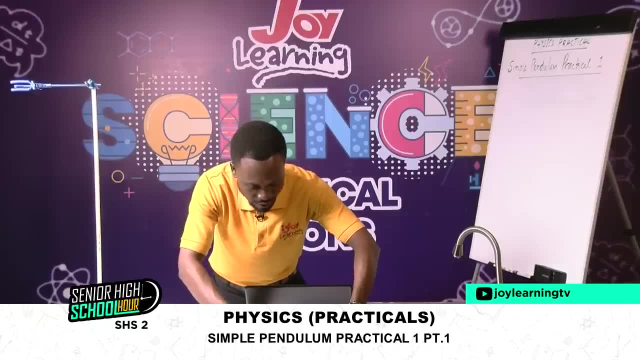 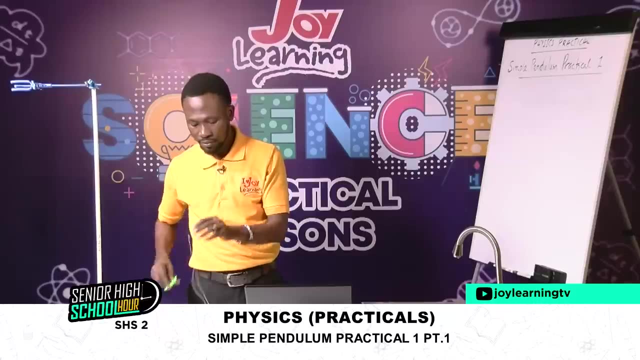 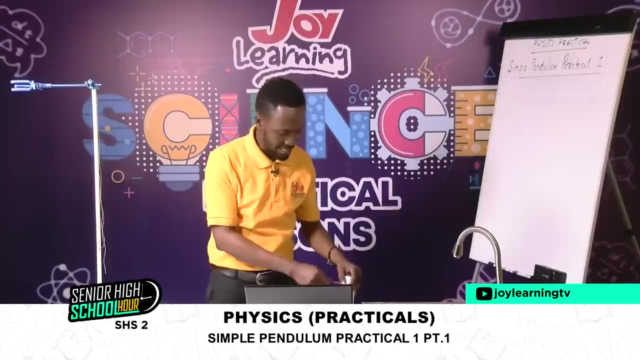 whenever you need it. it will help you to do that. so 120 cm long, that should be okay. so that is my thread. I'll just hang it somewhere so that I don't just lose it and I can put this bulk one aside somewhere. later on I'll get back to it. so I have 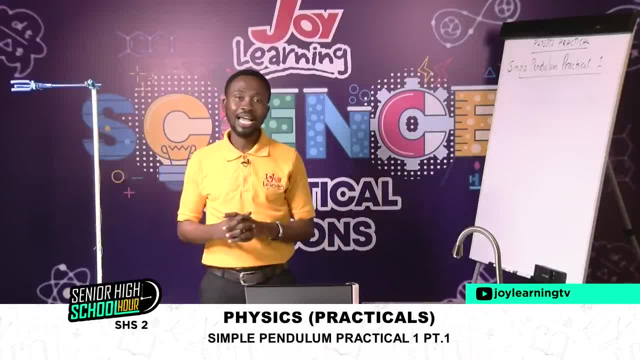 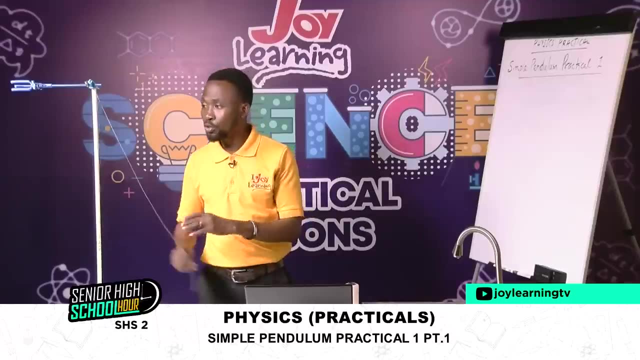 my thread 120 cm long. now the next thing: I'm asked to suspend the pendulum bulb, provided such that the length of the thread from the point of suspension to the middle of the bulb l equals 10 cm. so the best thing to do is to try to attach the bulb to the string. so I'm going to. 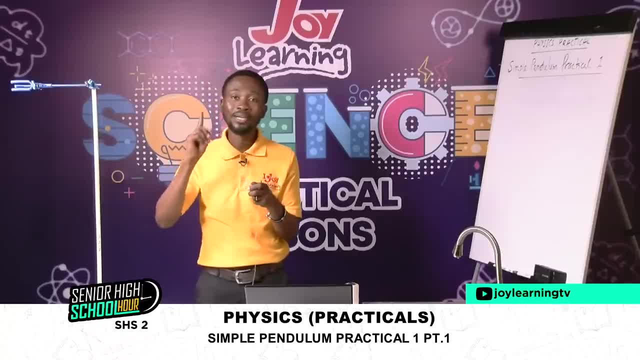 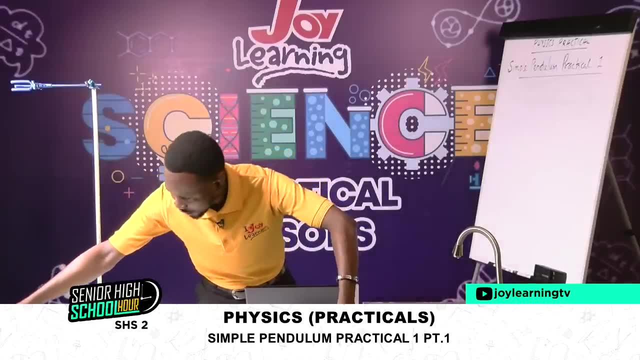 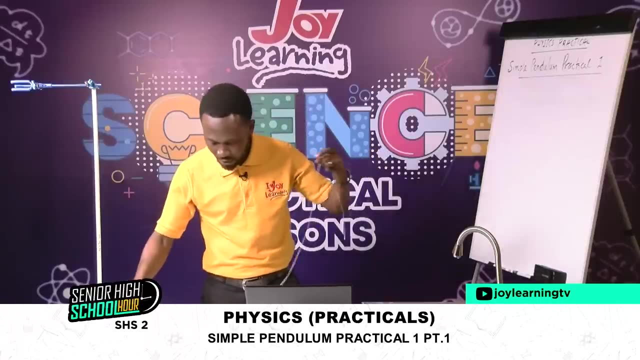 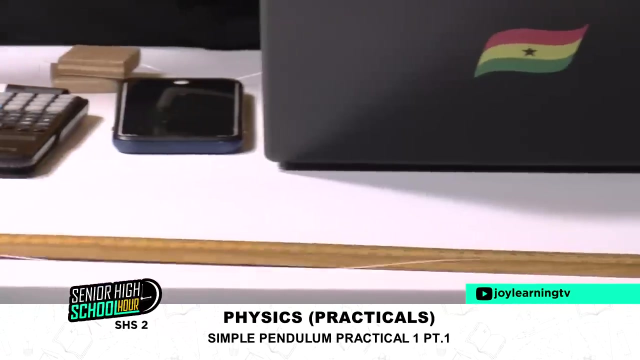 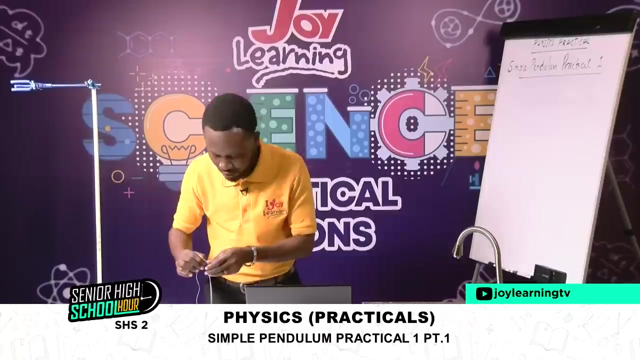 tie the bulb to the with string. so I'm going to tie the bulb to the string. so I'm going to tie the string. I will need only 100 cm length, but I have 120 because I'm going to tie the bulb to the string. That should be okay with us. So let me get my 120 and be sure of it, Okay. 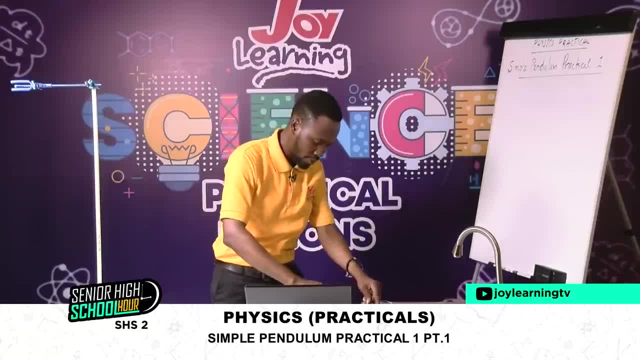 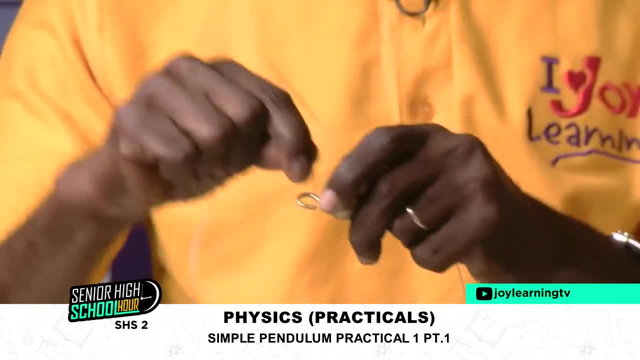 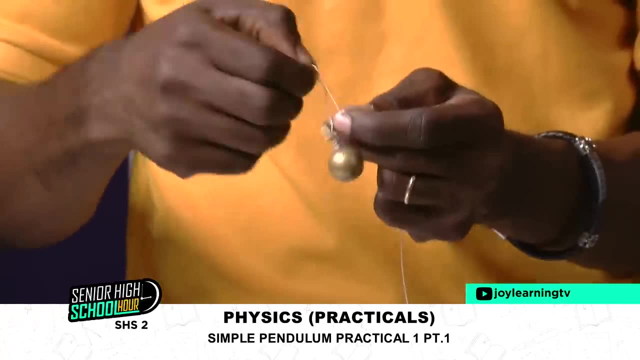 Then I will tie that to the pin. Okay, Then I will tie that to the pin. So I pick my bulb, I pick the string. Now be careful and tie and tie well, because if the string becomes loose and the pendulum bulb falls off, you have to start the experiment. 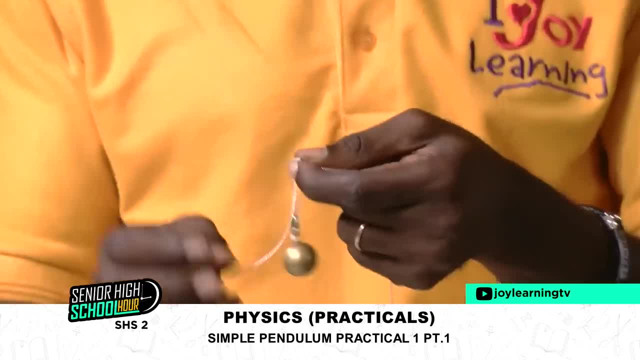 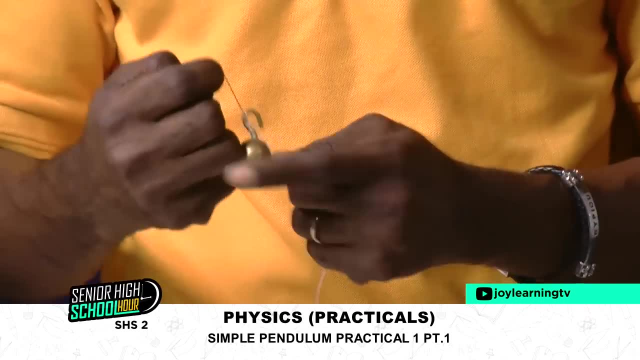 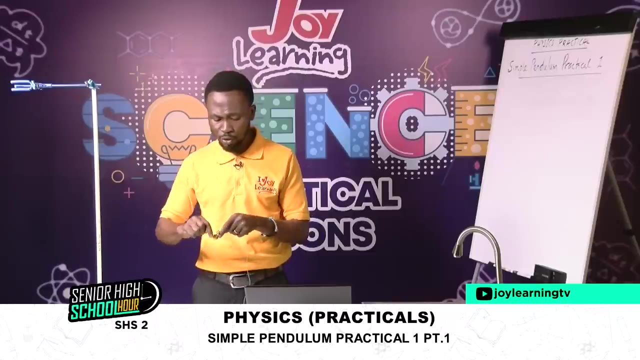 all over again, which will be disastrous, because I'm working with time, So I'm tying the string to the bulb and I'm making sure that I tie and I tie well, so that as I swing or as it oscillates, it does not fall off. So when you are through, you can try a little bit. 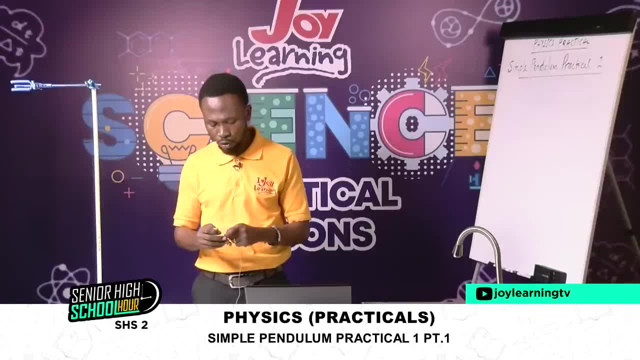 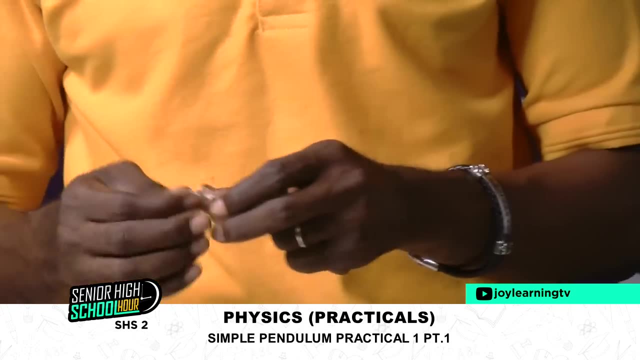 to see whether your bulb will fall off or not. There's a way you can do it and I'll show you in the GIFI. Okay, So I'm able to tie the bulb to the string. Now I'm going to swing it, So I'll try and see. if I swing this, will it fall? I mean basically there. 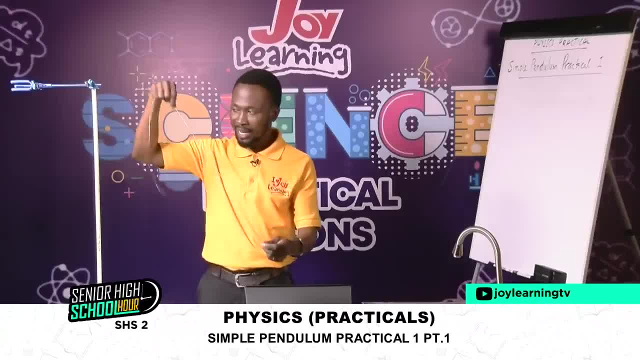 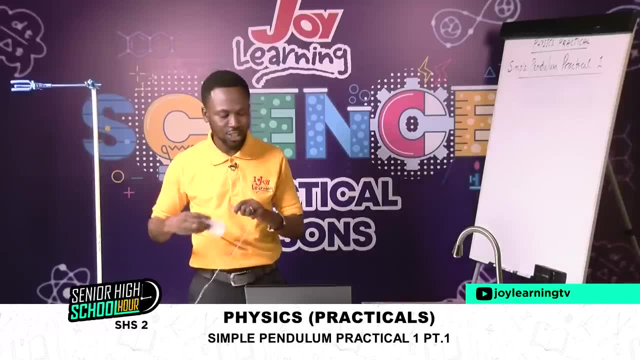 is some force. If it will not fall now, I'm very sure that when I suspend it and I'm swinging it it will not fall. So now I've tied my bulb to my string. Then it says that I should make sure that the measurement from the middle of the bulb to the point of suspension to 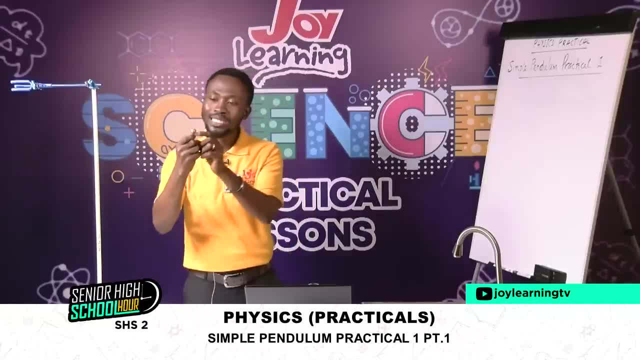 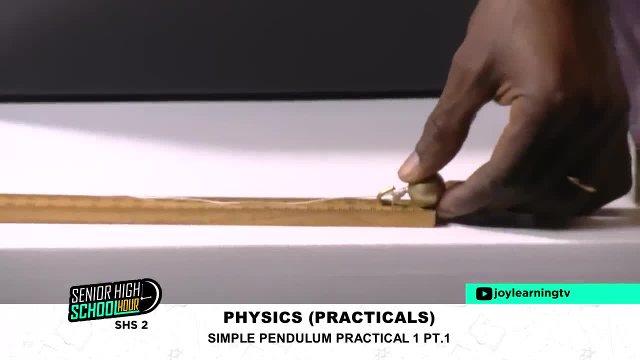 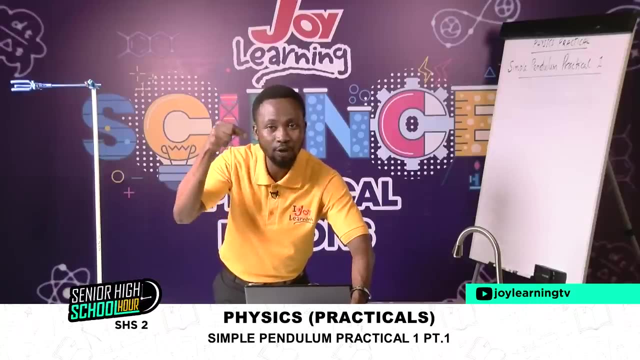 be 100 centimeters. So you pick the bulb, put the middle of the bulb at one end of the meter rule, So that's one end. Then I want 100 cm. Note this: We always measure the length of the pendulum from the middle of the bulb to the end. Okay, So I'm. 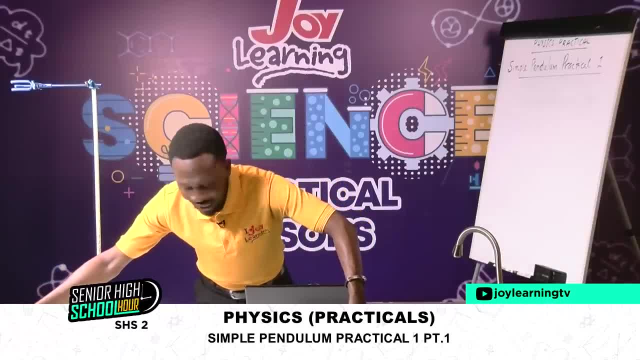 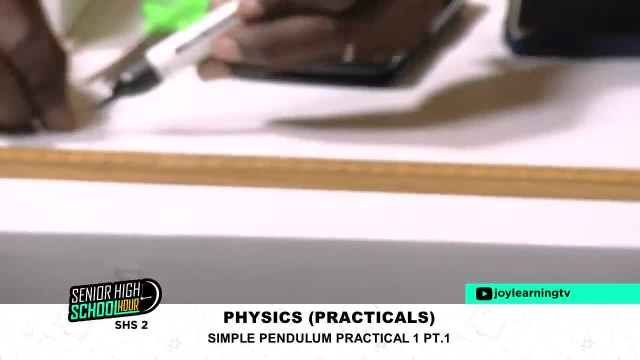 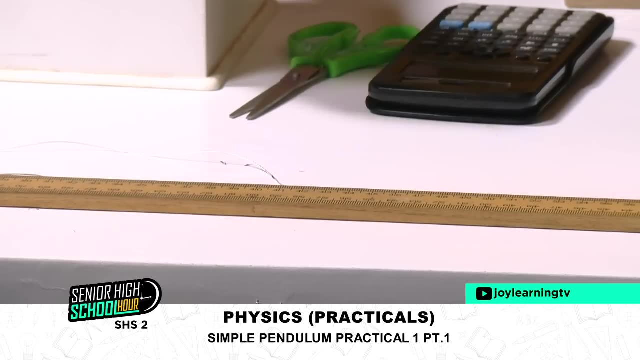 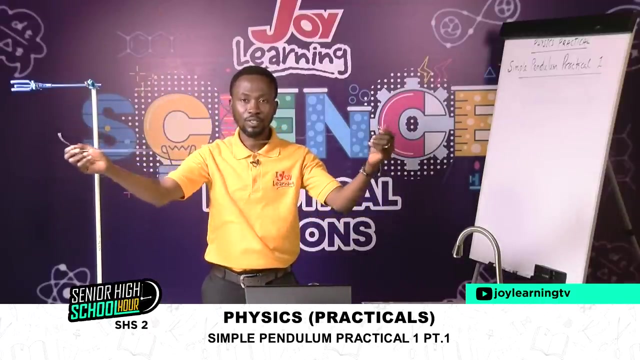 going to do that. That gives me 100.. 100 there. Then I'll make a mark at that point: 100.. So I have been able to make a mark at where my 100 cm ends There. Okay, So I've made a mark there. That is where I'm going to have my point of suspension. 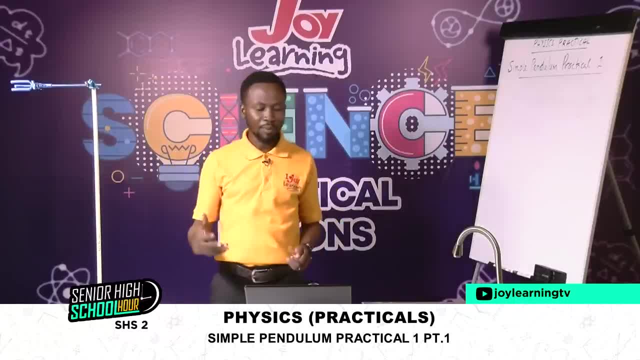 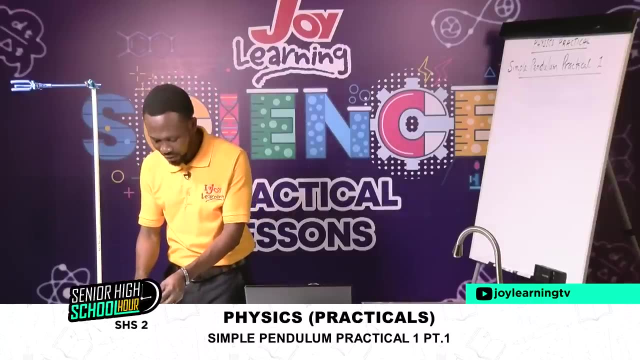 Now we move on. The question says that we should display the bulb through a small angle and determine a time for 20 oscillations. For the start, let me show you that. So let me just try, and then mount or fix it on the radar stand. So I'm fixing it there, These. 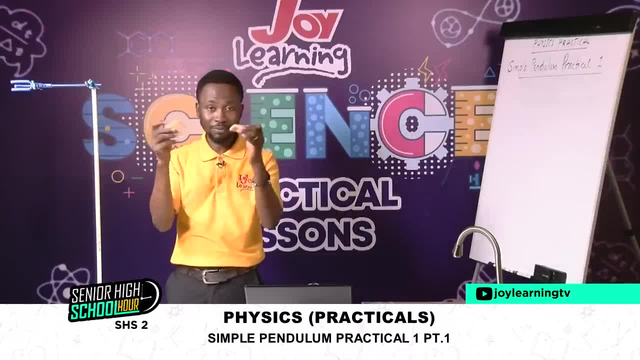 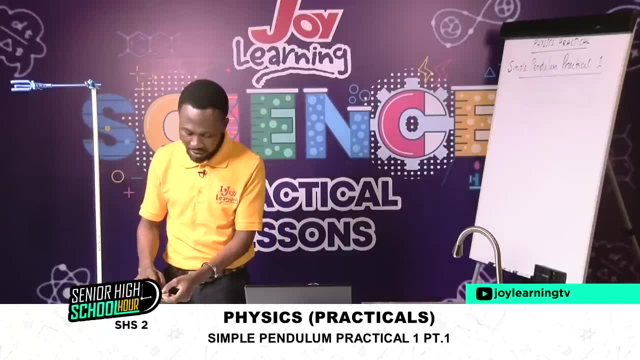 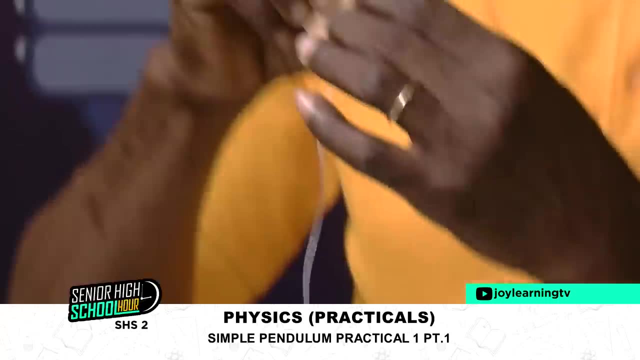 are what we call split cores, Split cores. They have to be splitted. You can have a core that is full, but this one is split cores. There's two wooden bolts or slabs. Then I put the thread in between the split cores and then I put them together. Then I take them to the radar stand and clamp. 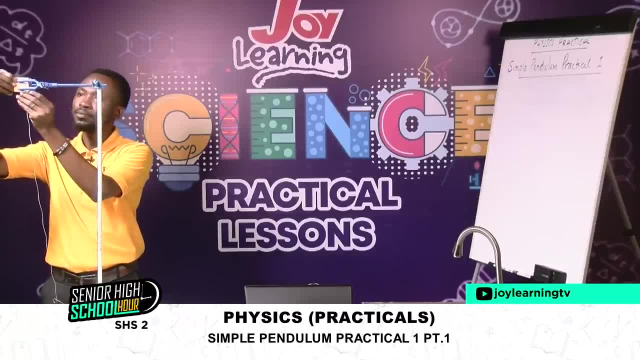 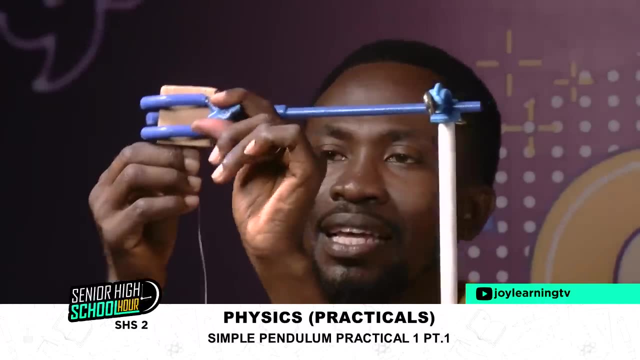 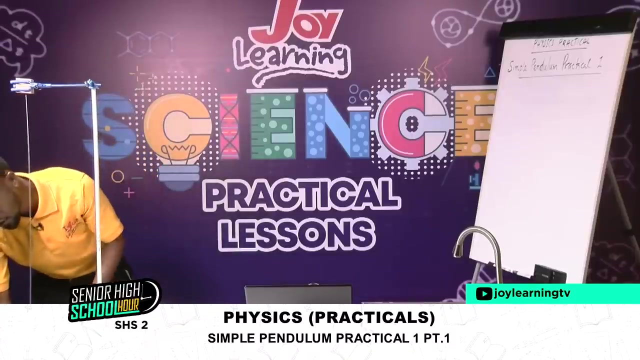 And then I try to fix it there Like that. Okay, Okay, Okay, Make sure that where I have my 100 cm length it's just beneath the split cork. Then the distance from that place to where the bulb is will give me 100 centimeters. I'm trying. 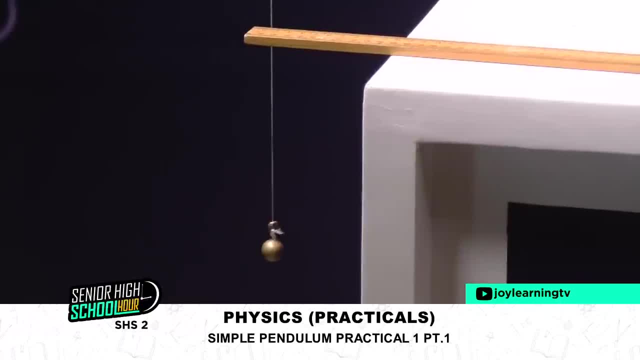 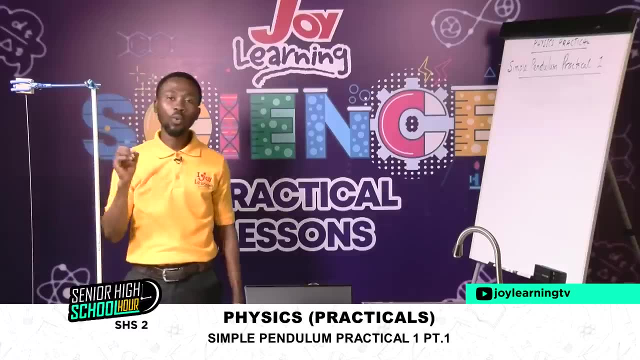 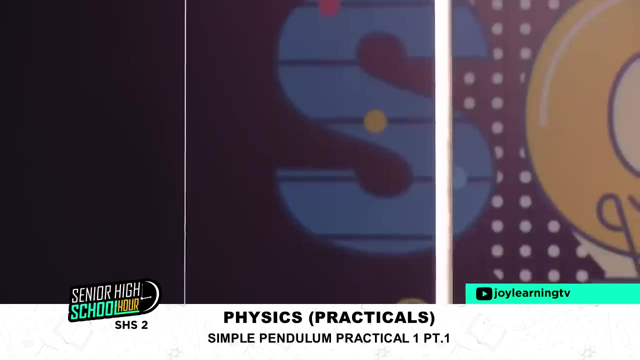 to show you something very important here. So from where I have suspended the thread to the middle of the bulb is giving us 100 centimeters. Okay, Boom, Okay. Now it says I should displace the bulb through a small angle and determine the time for 20. 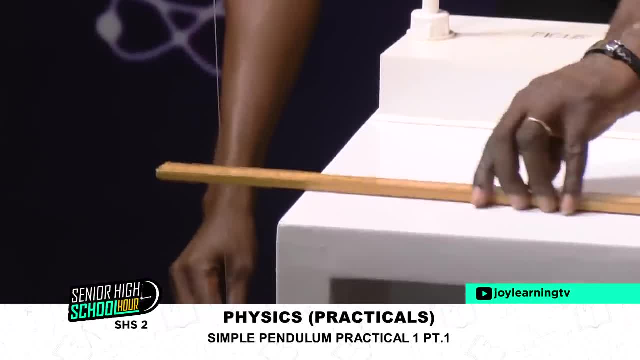 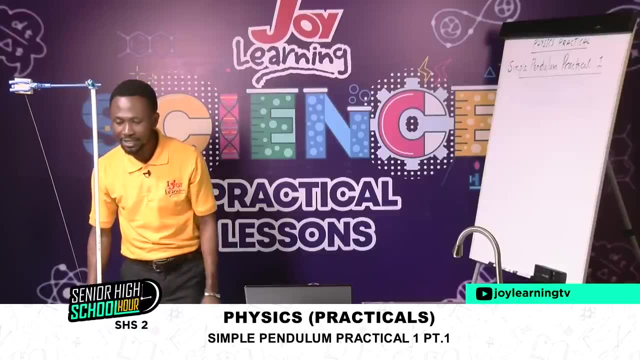 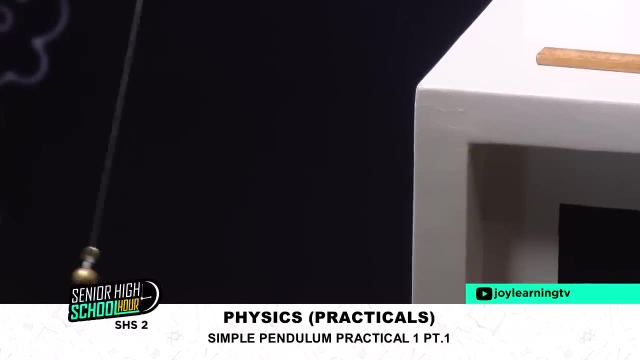 oscillations. So ideally I take the bulb, I hold it this way: a small angle of displacement, then I displace it, so I leave it for it to oscillate to and fro. Now an oscillation means the bulb starts from one point. it goes and comes back to that. 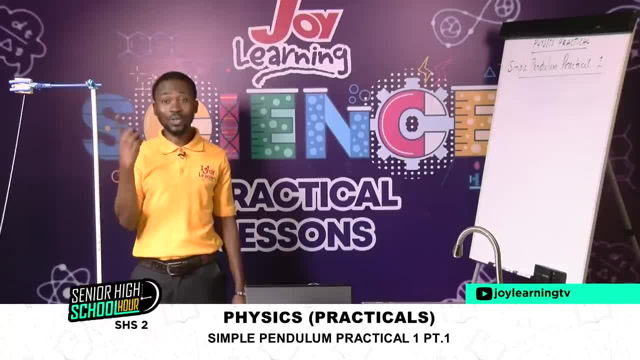 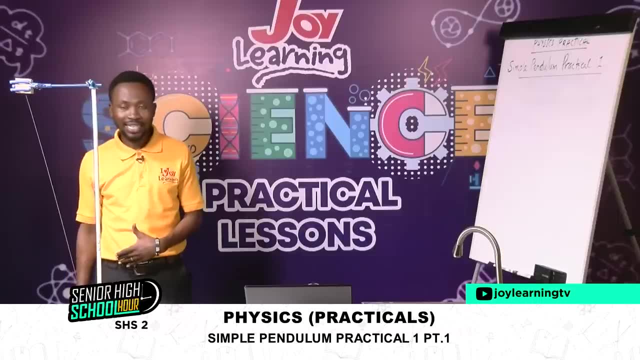 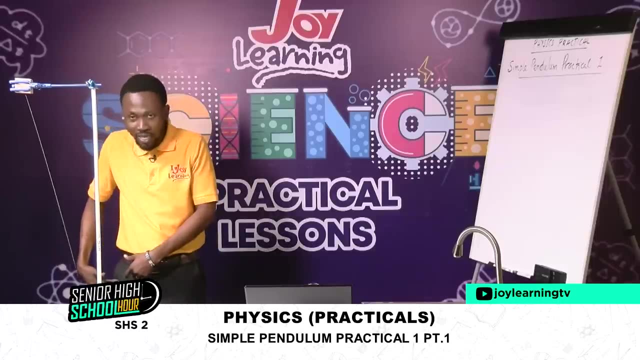 point where it began a movement. then that becomes one oscillation. So, assuming I have the bulb, I hold it. I displace it to this side, so close to me. this way, If I leave it, that means I've displaced it. it goes and comes back to me. that's when 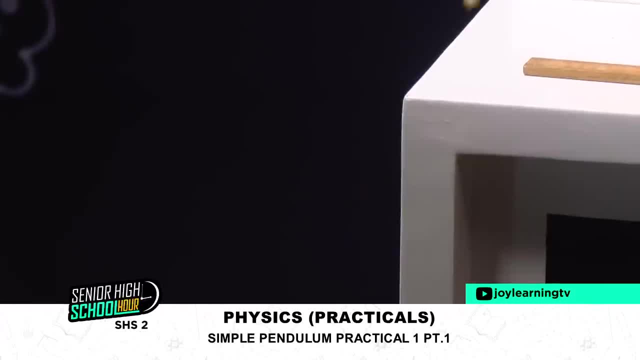 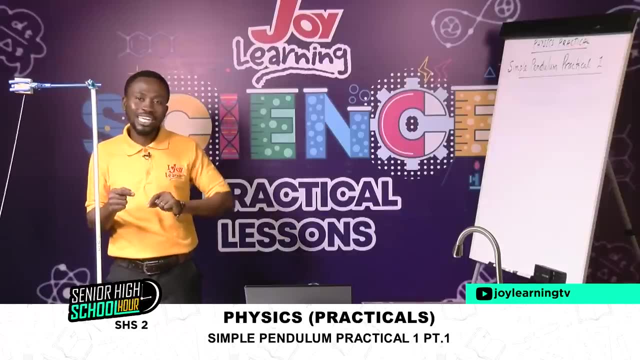 I say one, It has gone through one oscillation. So when it goes and comes back to me again, then I've gone through two oscillations. So an oscillation should start from one point, go and come back to the original or previous. 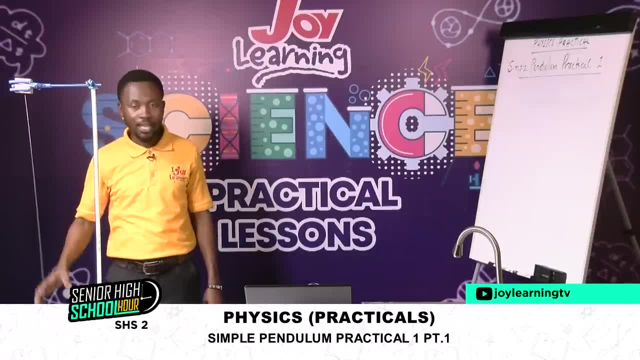 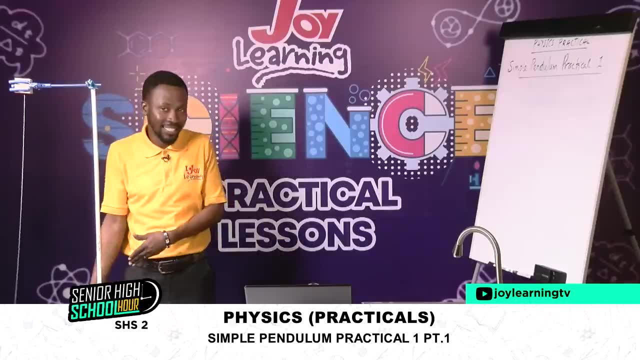 point before it becomes one complete word: oscillation. So you're going to do the oscillations for 20 times Simultaneously. you'll be timing it So as the bulb oscillates and you are counting, you are also timing it. 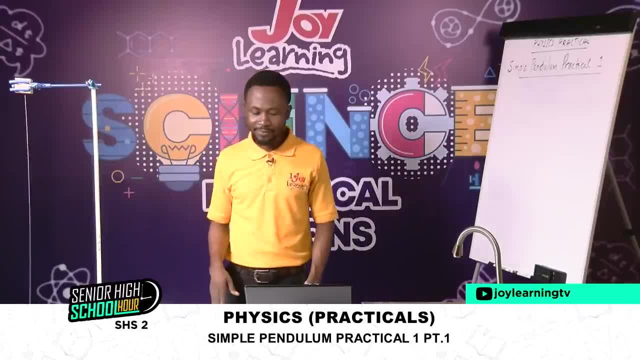 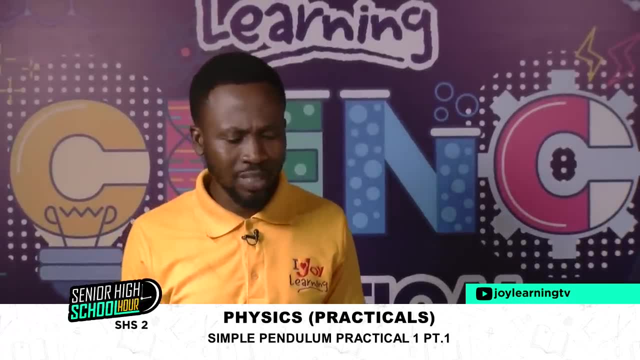 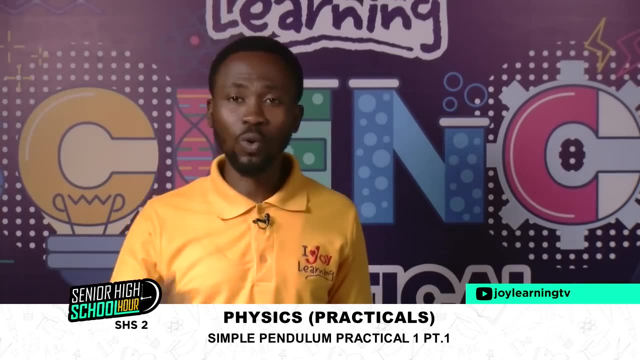 Then it goes ahead to the next oscillation. You have to say: calculate the period t of the oscillation, which we know how to do or we'll learn it pretty shortly. Then it says you should also determine t squared. Now it says: repeat the experiment with. l equals 80,, 60,, 50 and 40.. 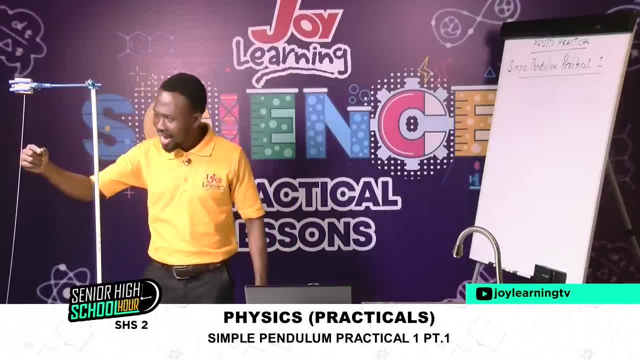 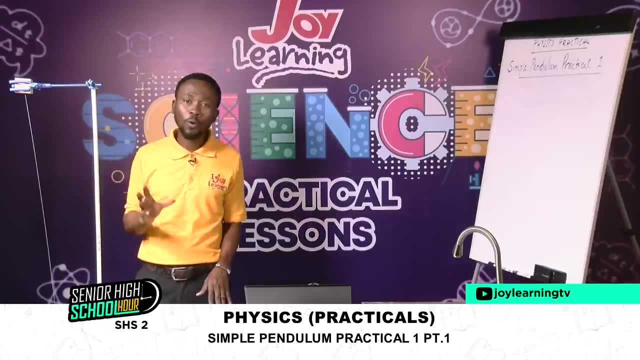 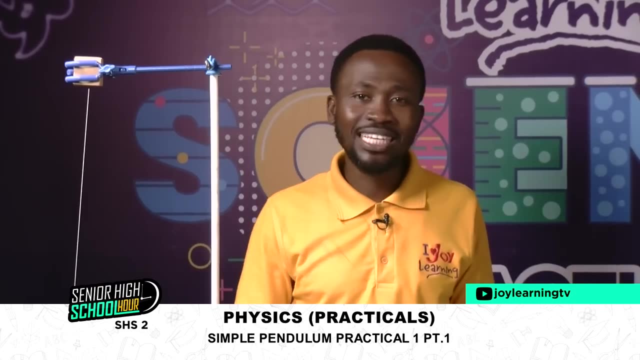 So it means that I have a length of 100.. I will oscillate and count for 20 oscillations. Now, another precaution for simple pendulum experiments is that whenever I'm supposed to do an oscillation, you repeat the oscillation for each length. 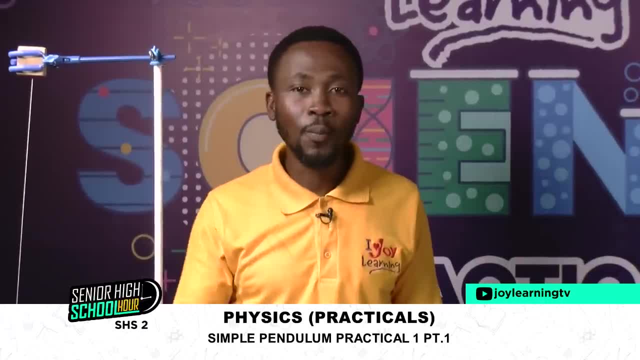 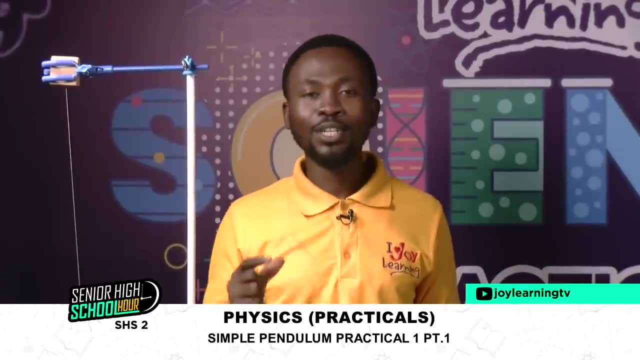 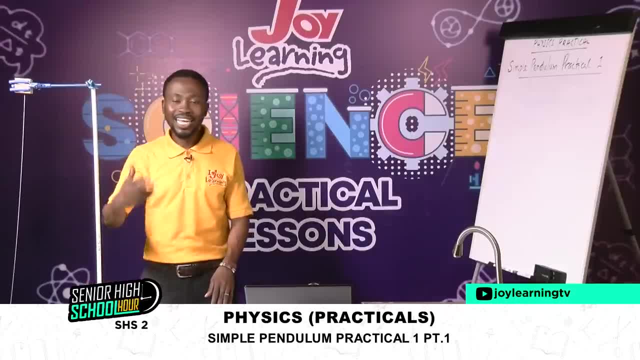 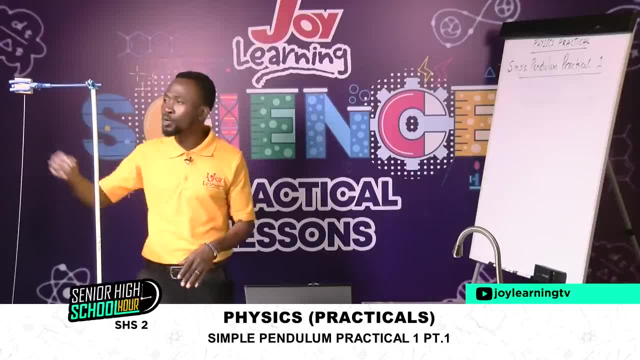 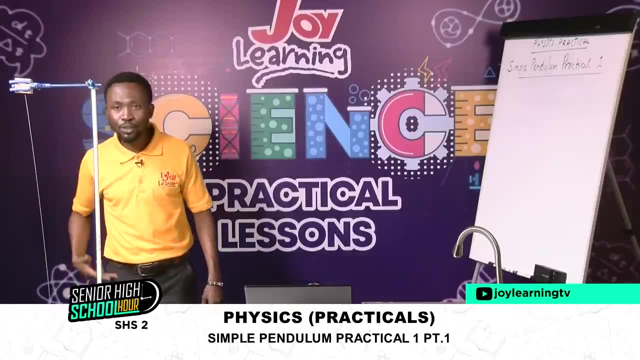 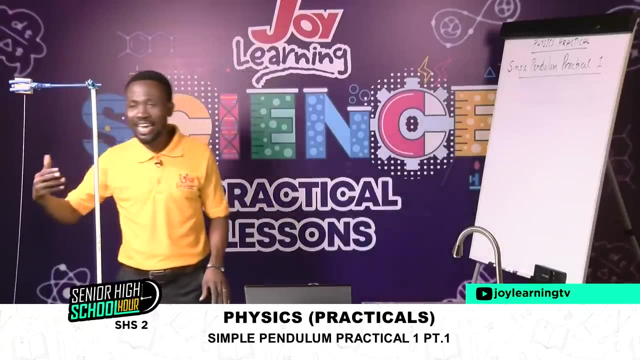 So do you have to now remove this? Can I measure 80?? Can I mount it here and oscillate for 20 times twice, Then remove it again? Can I measure 70, oscillate for 20 times twice and move again? 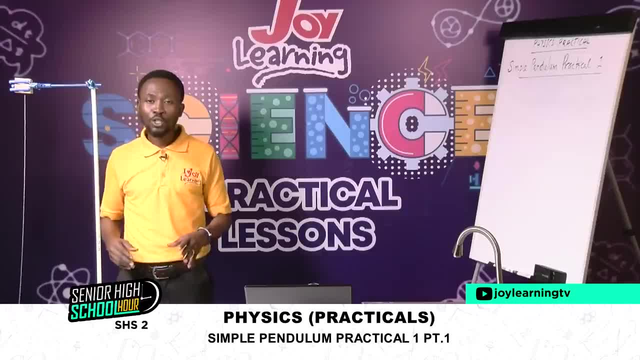 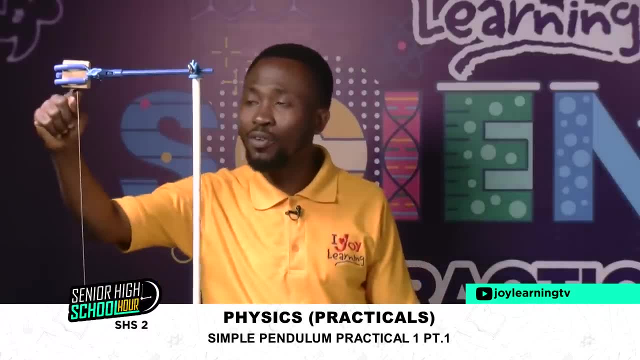 No, that time will go against you. So that is why I'm saying: read through all the questions before you start working. So from the question I will need a length of 100.. Then I will need a length of 80.. 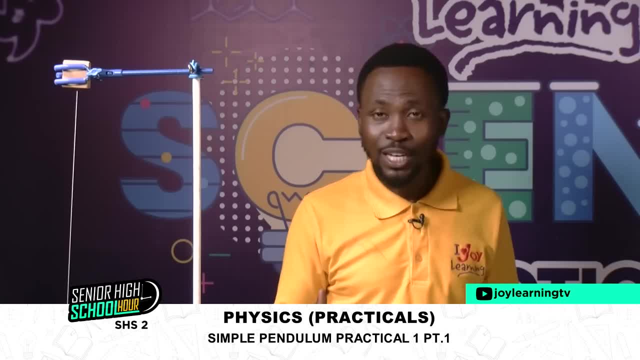 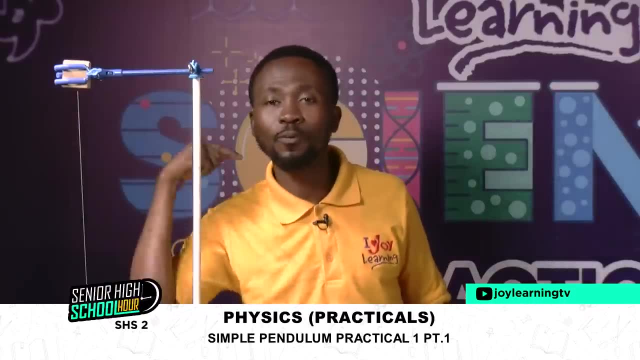 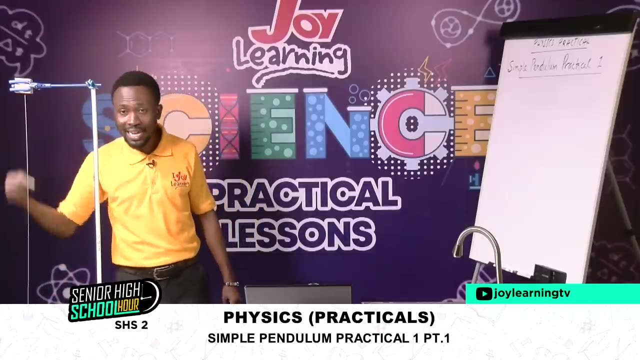 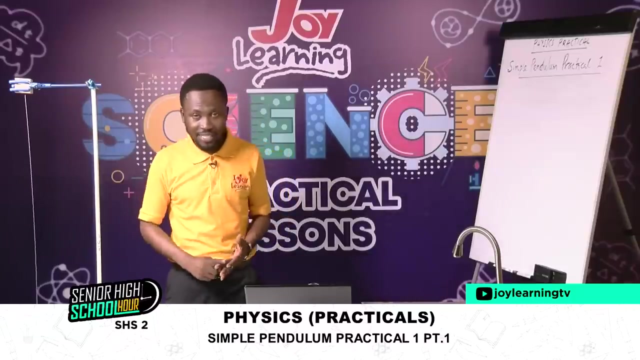 Then 60. Then 50., Then 40.. So the best thing to do is that you measure all these lengths first before you suspend the pendulum ball- Very important. So I'll go ahead and measure for 80,, 60,, 50,, 40.. 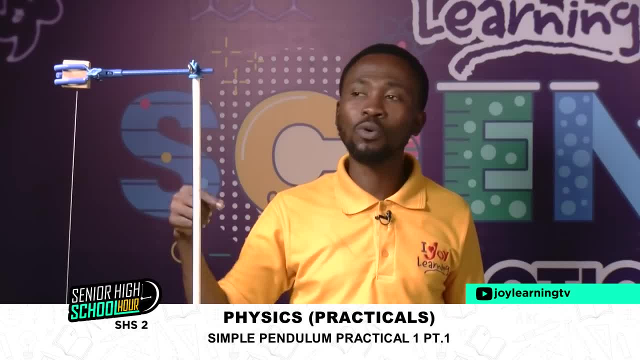 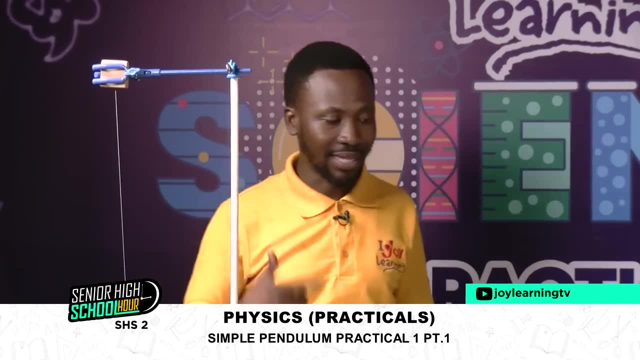 I'll do all that before I suspend. So all I'll be doing is that whenever I need any length, I'll just remove or loosen it here and then pull it up to that length. Then it says that we should also calculate our results. 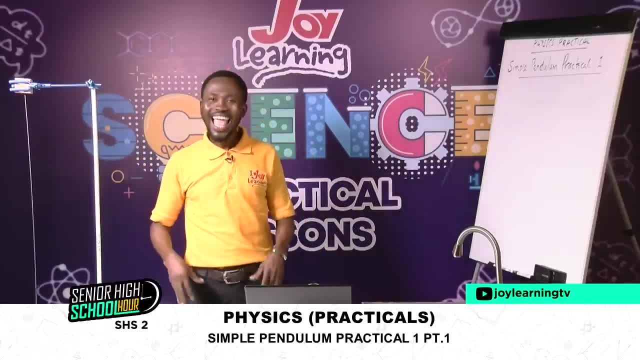 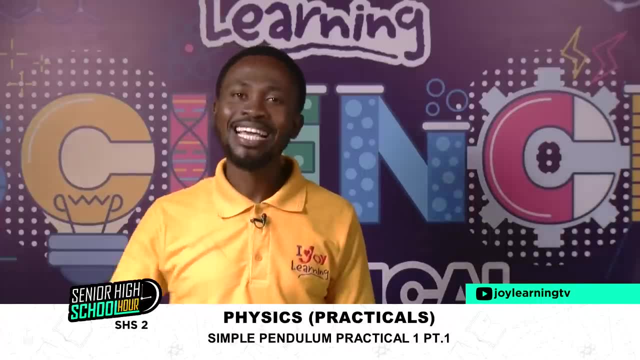 In fact, in the physics practical work, every practical work, you'll be asked to tabulate your results. Very important, In fact, it is one of the most important things in the practical work: the table of results or the table of values. 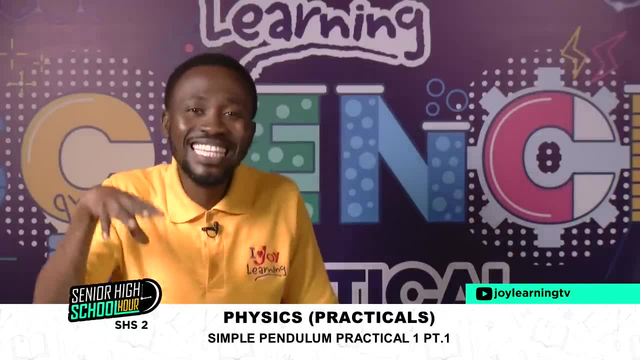 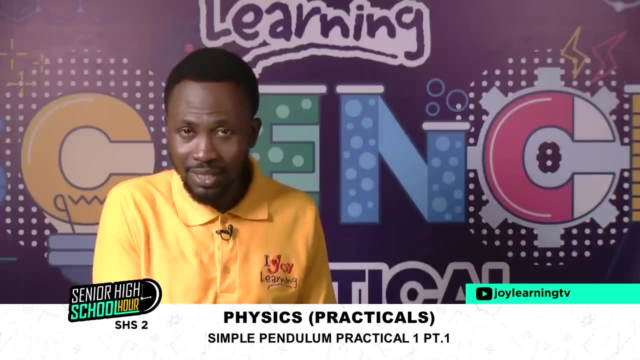 Why The examiner is not or will not be in the lab as you go through the practical work. So what is the evidence that you went to the practical work? It is your table of results. The table of results will show us that you actually went through. 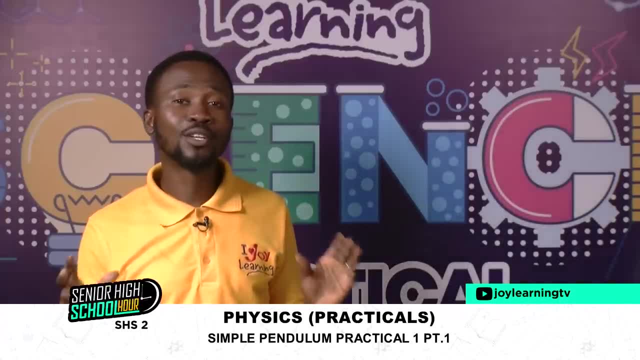 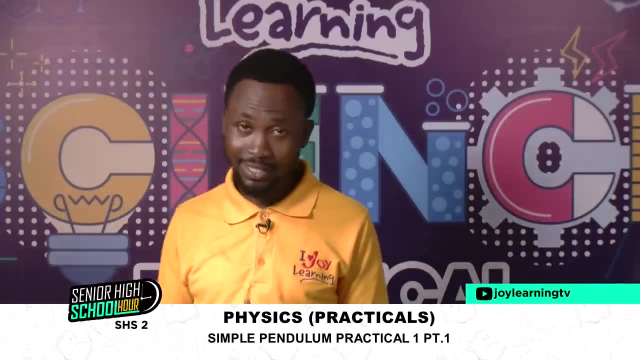 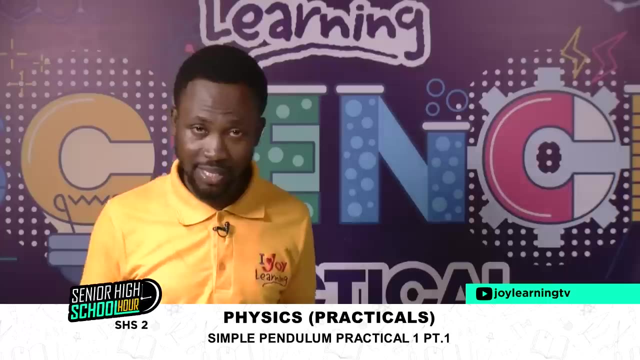 the practical work, The practical work, The practical work. Now there are some things to take note In the table of results. you don't have to cancel anything. Yes, If you should cancel anything, it presupposes that you cheated or your values were not genuine. 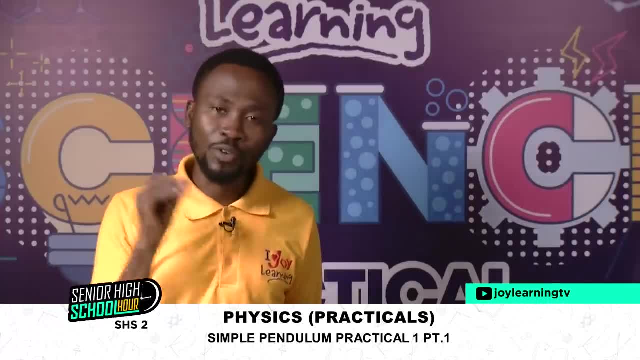 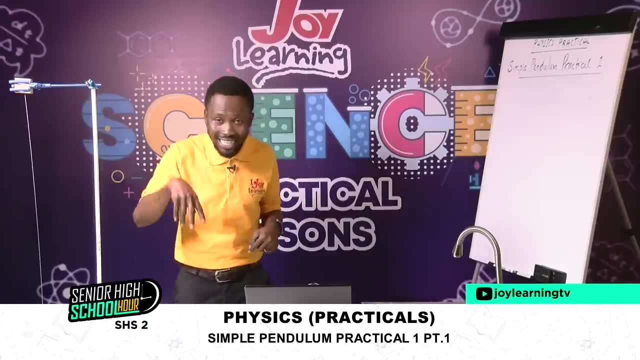 You didn't go through the experiment by yourself. So in your table of results you don't cancel anything. Now you don't also deepen or shade in. You shade values in the table of results. You don't do that. It should be neat. 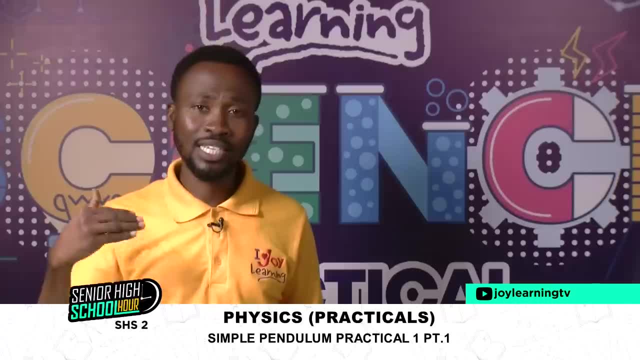 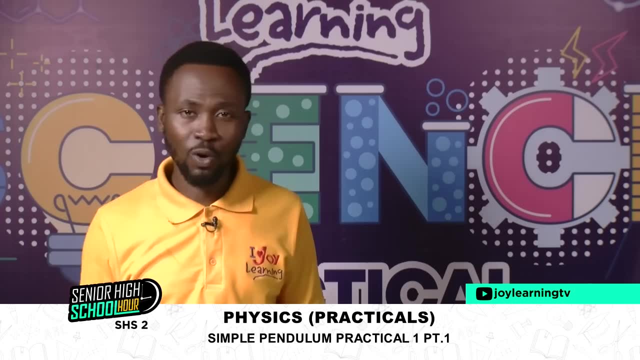 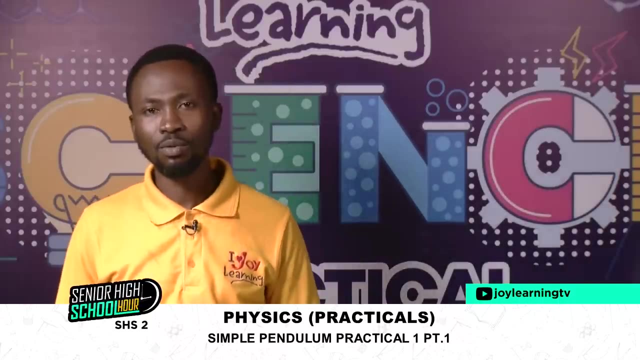 You write everything once and for all, So I'm going to show you how to do the table Now. it is always advisable to draw your table first before you start the experiment, because as you go through the experiment you get values. Then you put the values into the table. 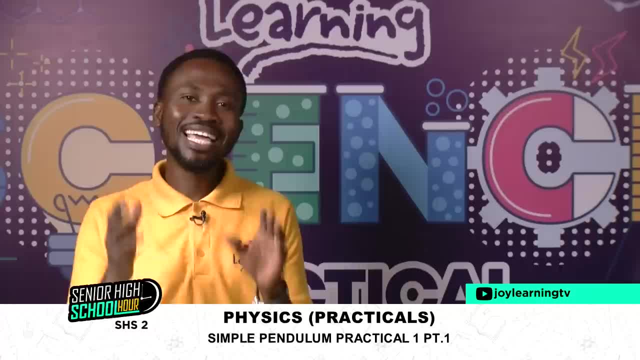 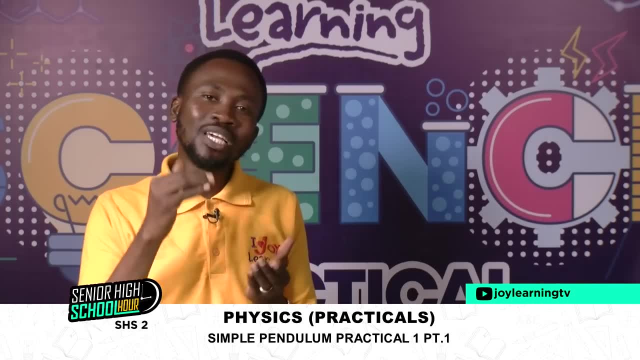 Very important, So I'm going to draw the table with you Now. each experiment counts with its own table, So there's no fixed table for all experiments, No, So whatever you give as headings in the table comes from the experiment. 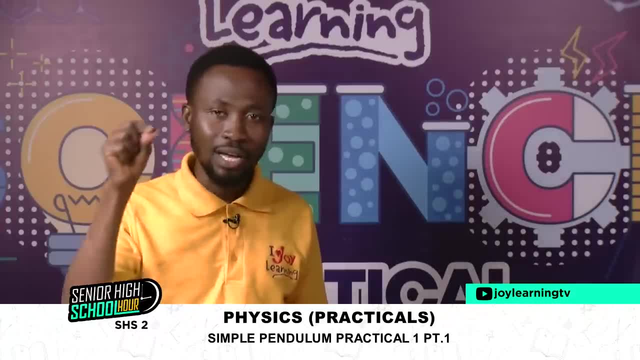 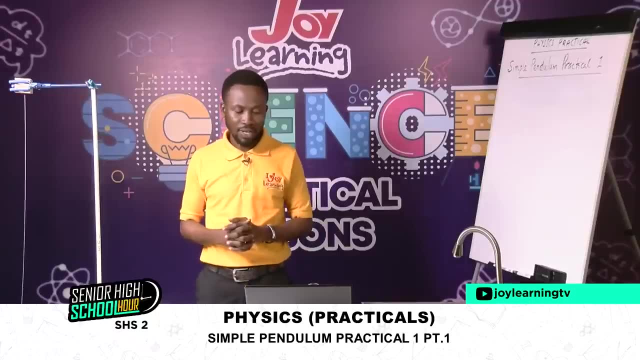 So you read the question and read very well, Look at the things you are asked to put in the table or you need to put in the table, and then you do that. Then you are asked to plot a graph, which will be another lesson altogether. 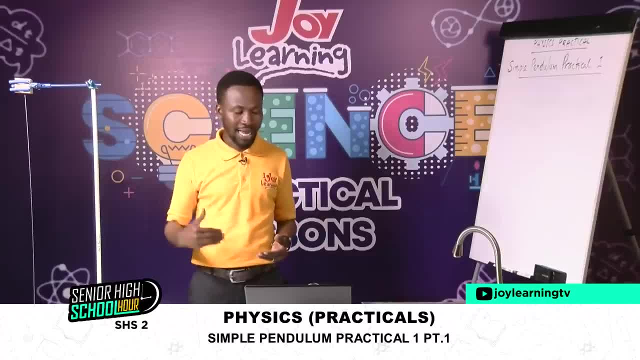 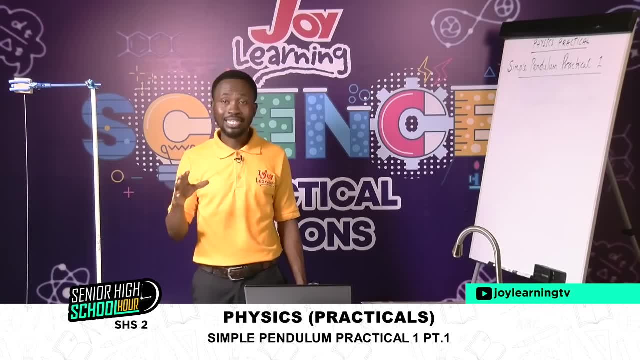 So we are going to focus on going through the experiment and then drawing our table. So let's begin with the table. Now you go to the question. It's question number five, That is, tabulate your results. So I'll go and say question five. 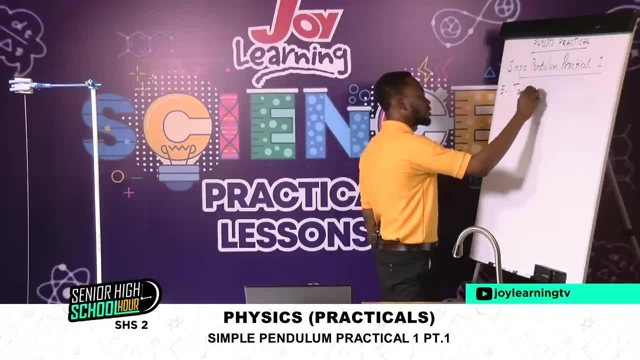 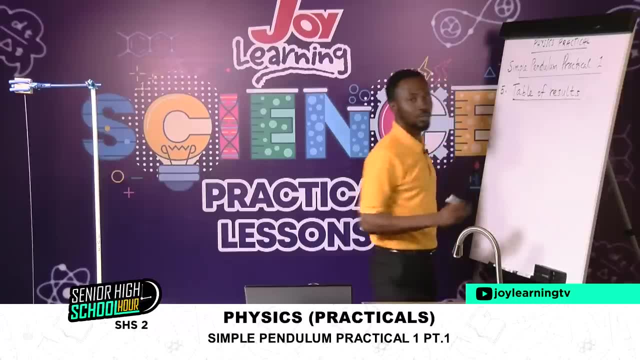 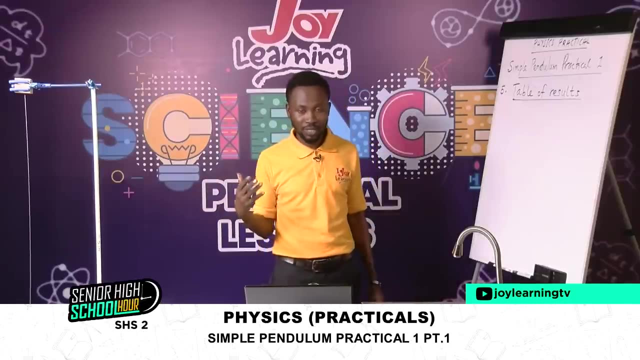 And I'll write table of results And I'll underline it And that text will say: table of values. Same thing, Table of results. Now what and what will come in a table? Anything you're going to measure, that varies. 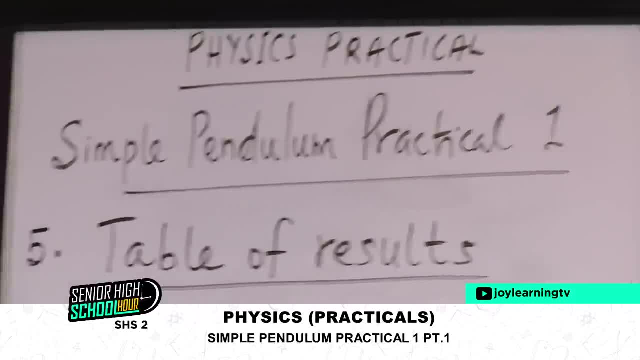 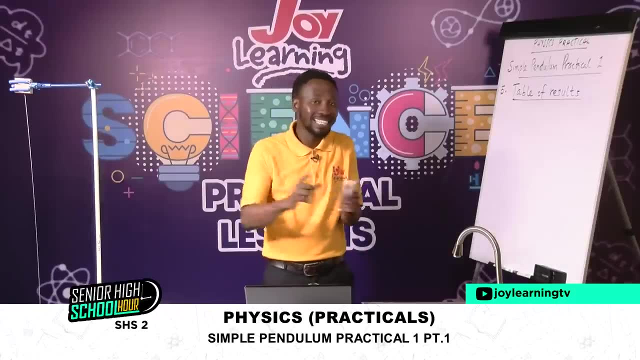 That is different, And anything the question asks you to evaluate or measure and record, And then anything that I'm asked to plot on the graph, plot something against something. those things will come in the table. Now. it says that we should get length L. 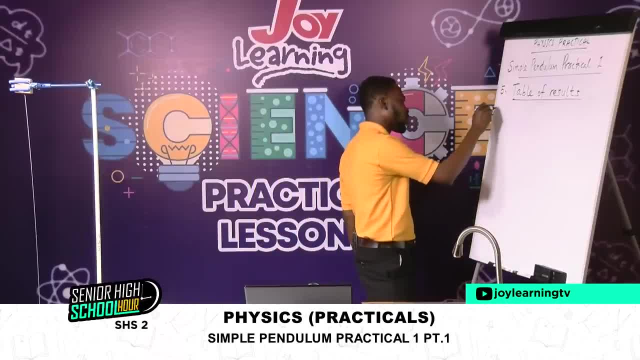 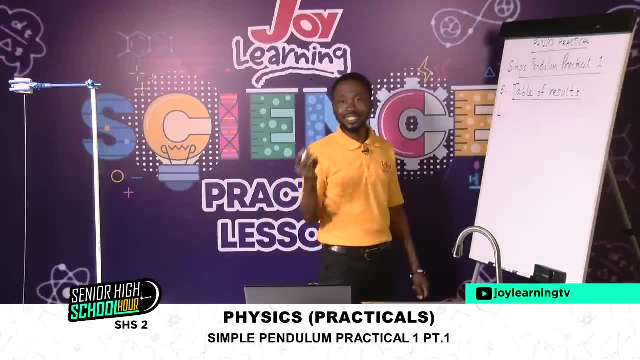 So I'll write for my first column. I'll put L, capital L, because the question gave capital L. So now, what's the unit of measurement of the length? According to the question, 100 centimeters, So it is in cm. 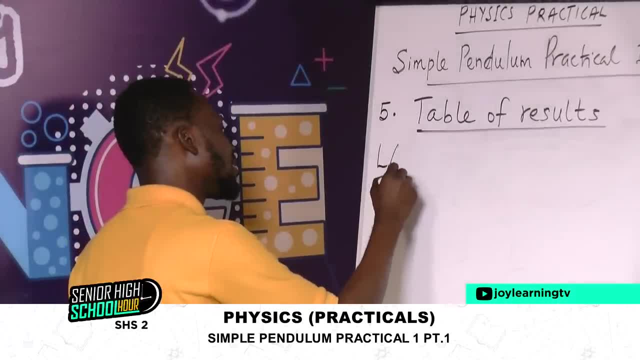 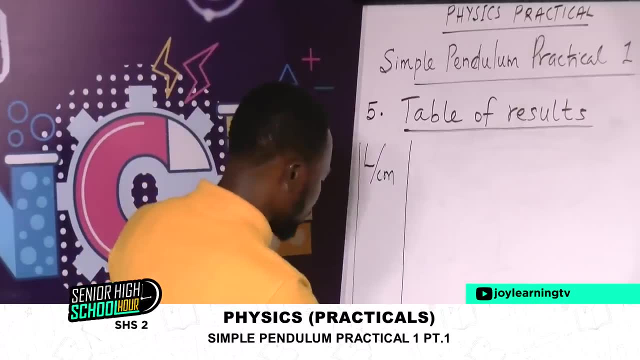 So I'll just put here stroke centimeters. That's for my first column. That's for my first column. I don't want to exhaust all the space I have, So let me just manage this very well. So that will be for my L. 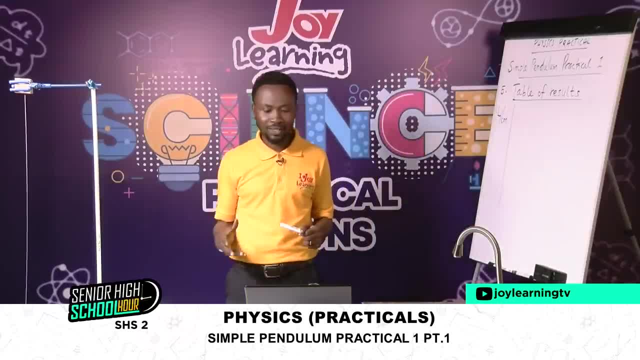 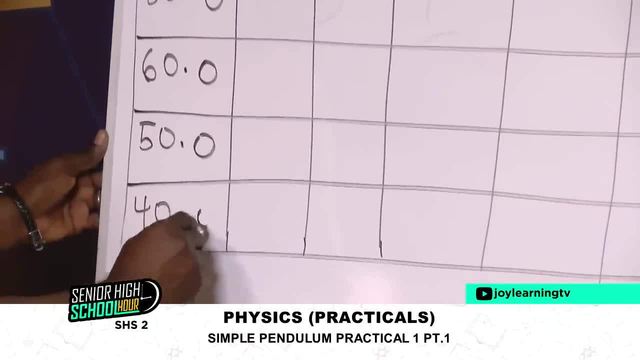 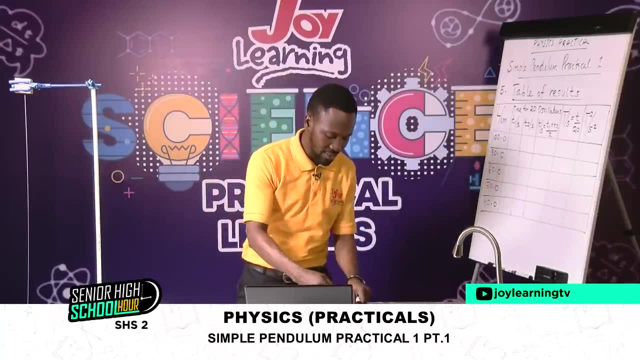 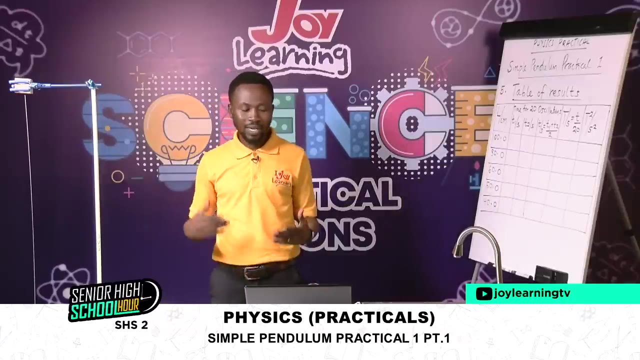 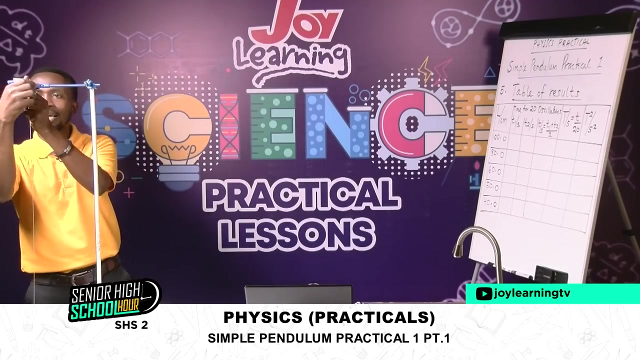 point zero, point zero and then point zero. now you are good to go. now your values are precise and you will not be penalized for not putting decimal places in there. so we go back to the question. we need to get a length: 180, 60, 50 and 40. so i've told you, don't mount it and be removing. 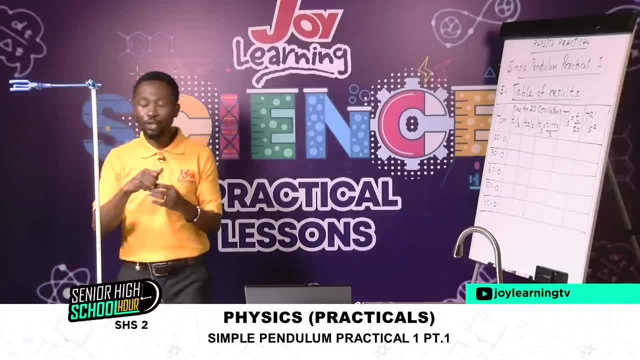 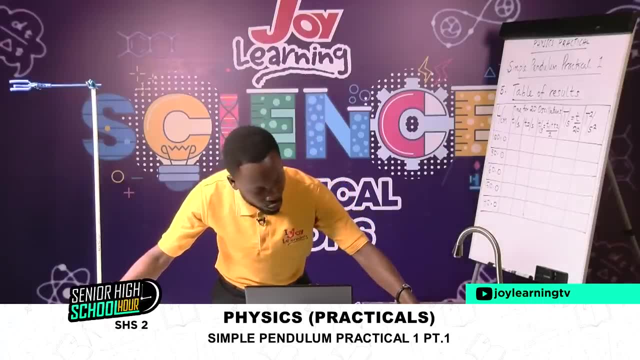 it from time to time. no, get all the measurements first before you mount it once and for all. it will save you time. so i'm going to start. i've already have, i already have my hand read which is there, so i'll hold the bulb at one end, then from the middle, i need 80, i need 80 so i get to the. 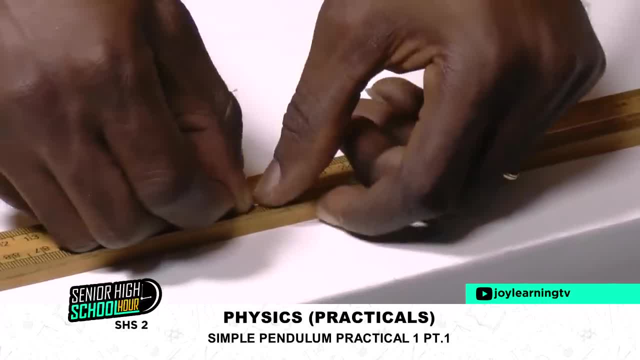 rule. that's where i have my 80 and then i can make a mark at the 80. you can use your pen to do that, so i have my. you can use your pen to do that, so i have my. you can use your pen to do that, so i have my. 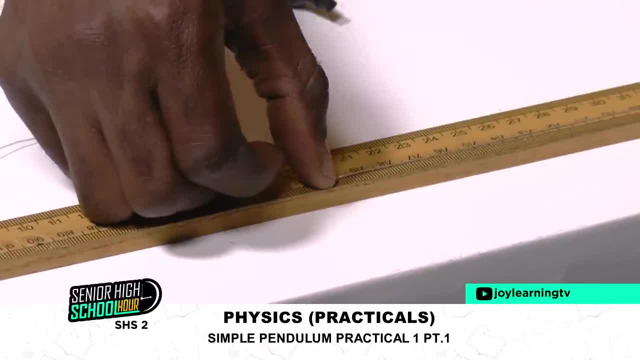 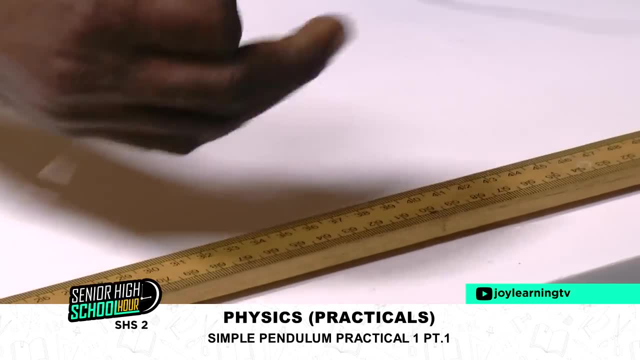 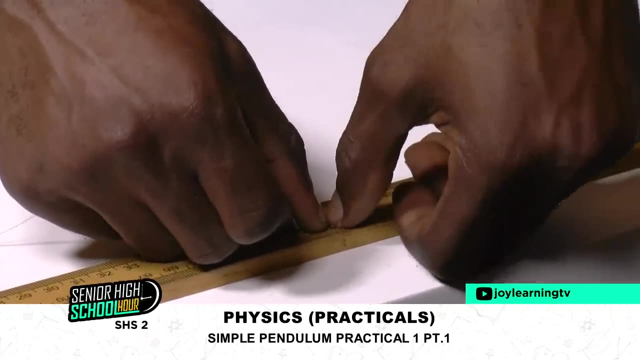 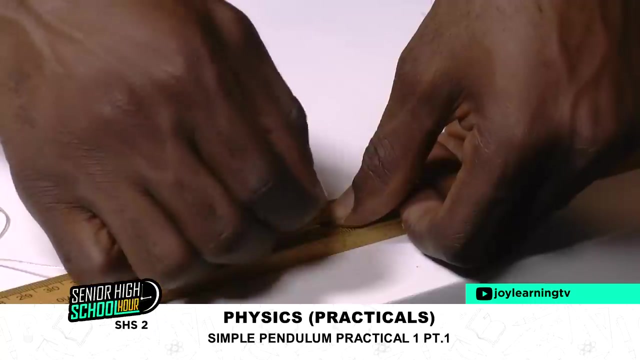 there 80 from 80. the next one i have is 60. good, so i i hold the thread and i come to 60 and that is my 60 there. i put my thumb there firmly, then i put my marker, i take my marker and i put a mark there. so i have 60 from 60. what we have is 50, so 50 is just here. 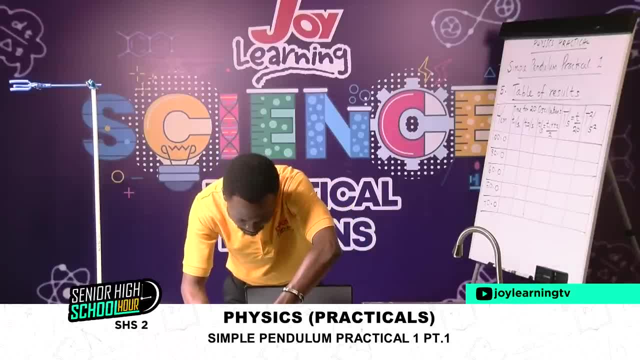 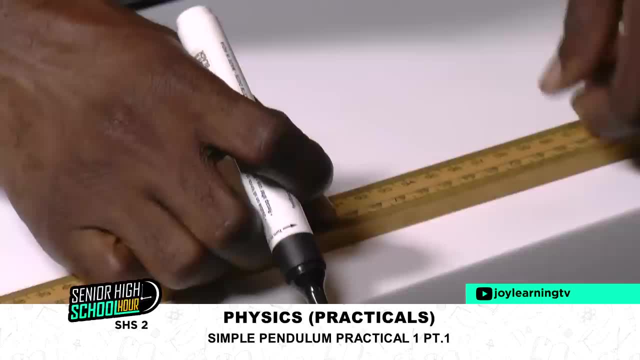 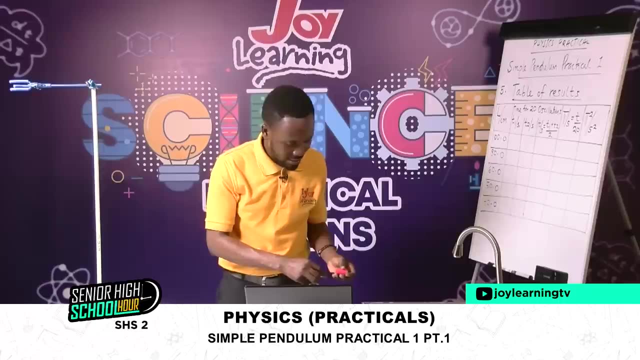 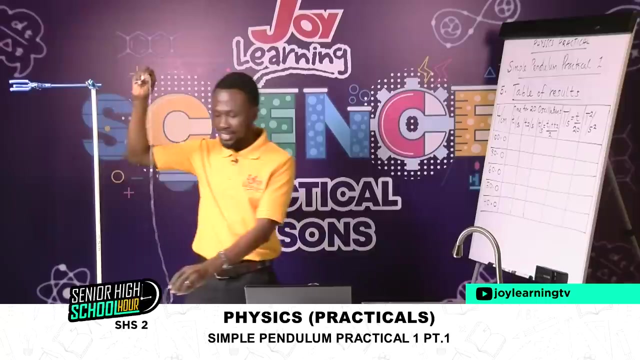 so i have 50 and i make a mark from 50. what we have is 40, so i get 40 and i make a mark there. good, so now i have all my marks in place for my lengths. so i have 180, 60, 50 and 40. now i can. 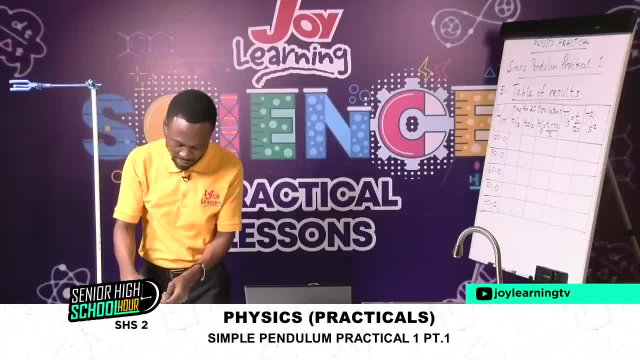 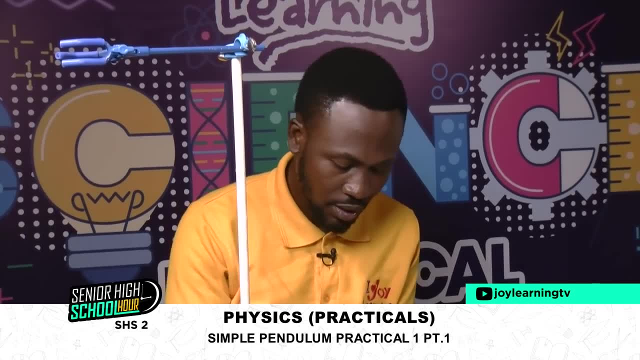 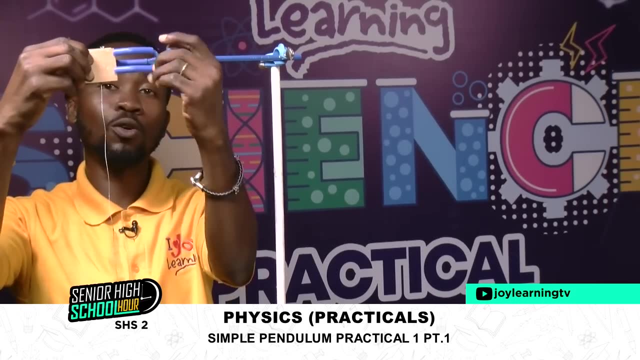 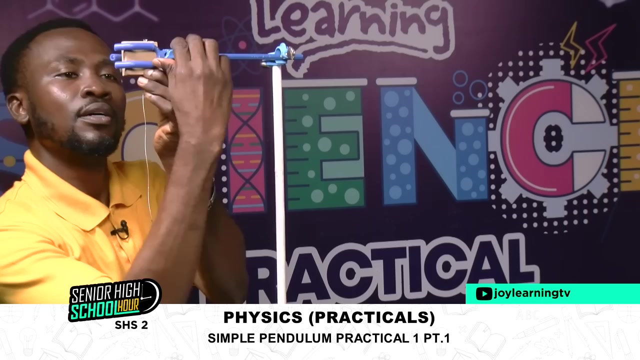 confidently suspend it from the rate of stand. mind you, my hundredth mark will be the last mark on the thread and it should be just beneath the split cock, right beneath the split cock. it should be quite firm so that it doesn't fall. if you fall, to pick it up. 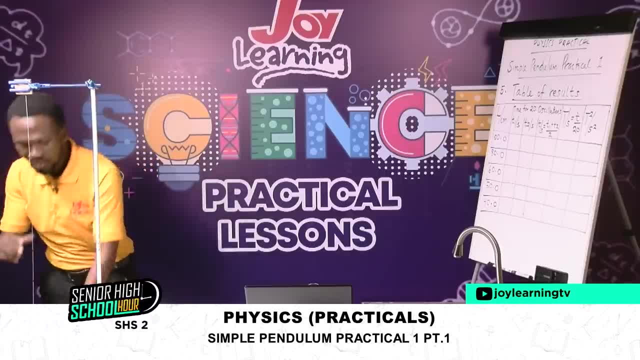 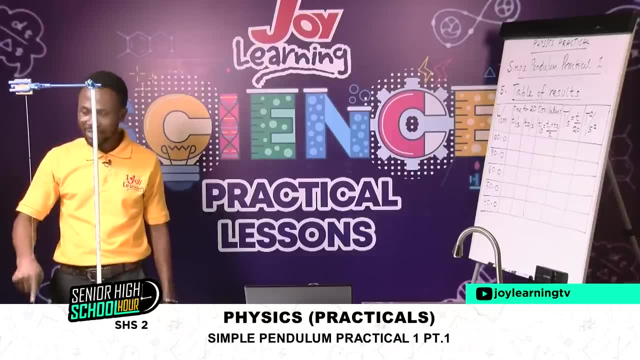 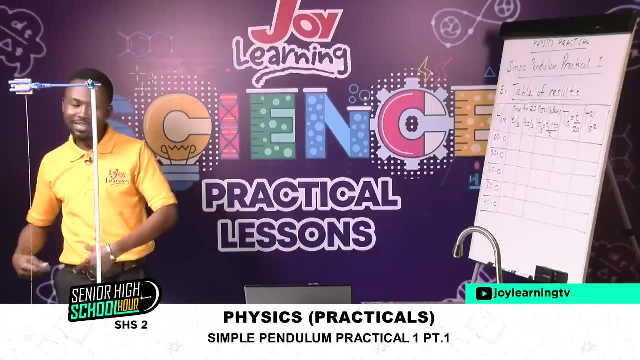 so let's see good, good. so i have my hundredth mark, 100 mark, 80,, 60,, 50 and 40.. So you see, I don't need to remove the thread. Go and measure, come back and mount, oscillate finish. 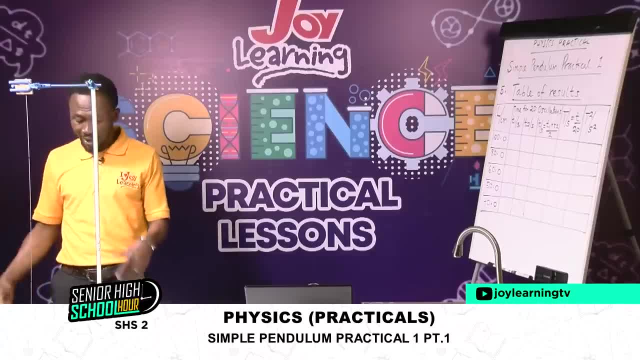 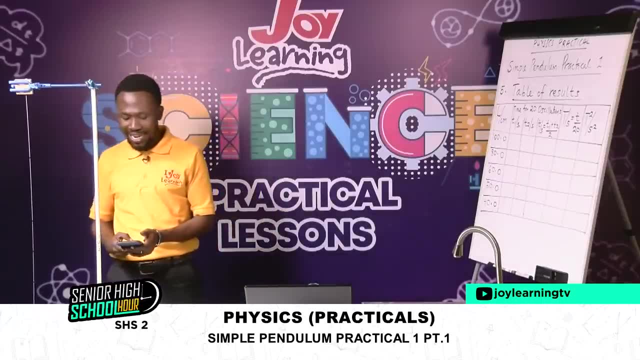 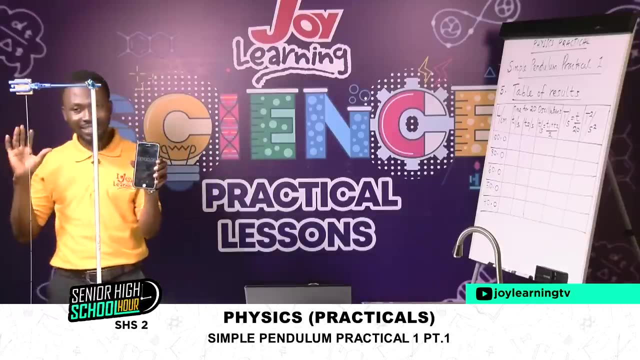 Go and measure, come back and mount, oscillate again. No, I have it all once at a go. Then I'm supposed to oscillate. Now I need 20.. Take note that on your stopwatch you have 0, 0, 0, 0.. 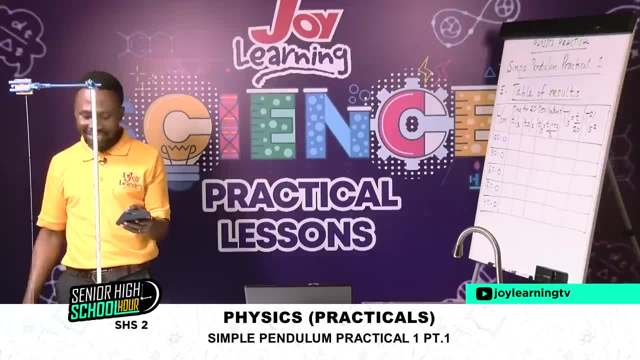 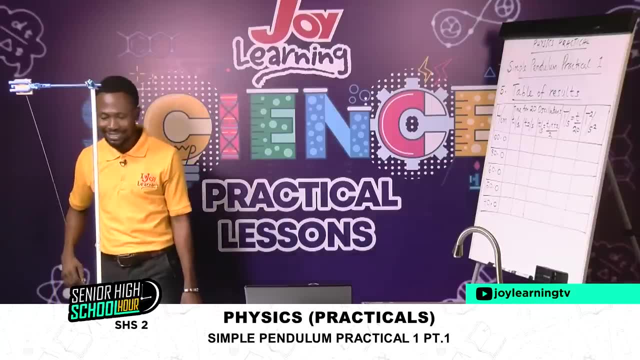 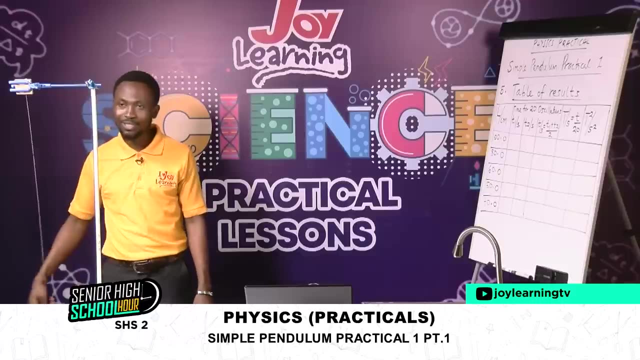 Everything is just 0. So as you hold the bulb I said don't displace it to a very large angle, Maybe like this: See what happens As it goes and it comes with time. the oscillation will not just go as it's going. 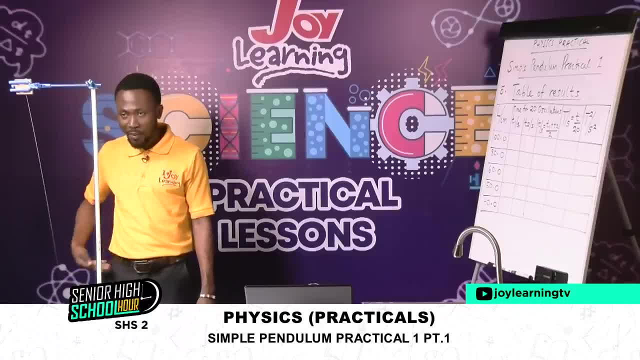 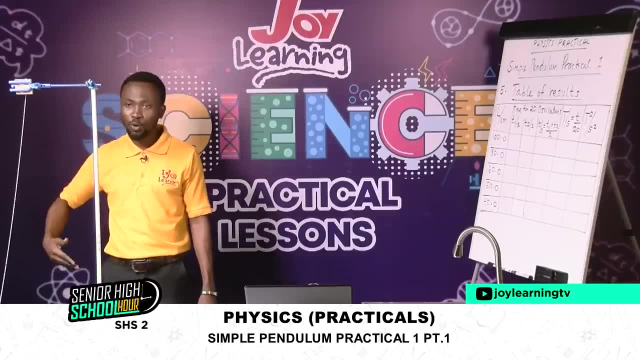 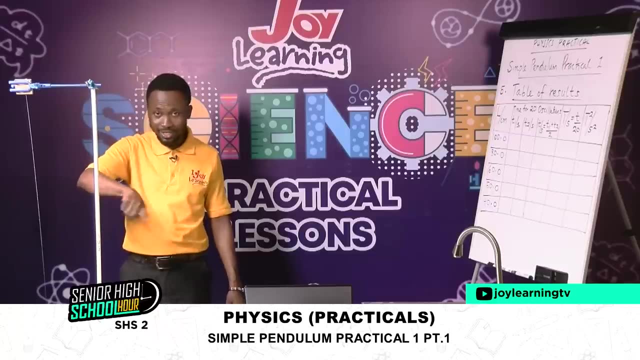 You will find the bulb moving and describing a circular path. We call it elliptical oscillations. So if you are not careful, the bulb will not go just as it's supposed to go: up forth and back like that, Rather, it will be moving in circles. 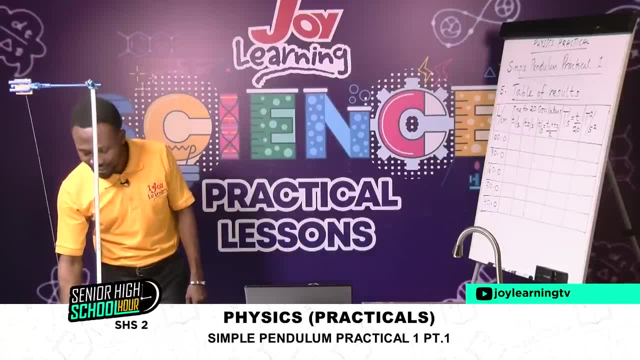 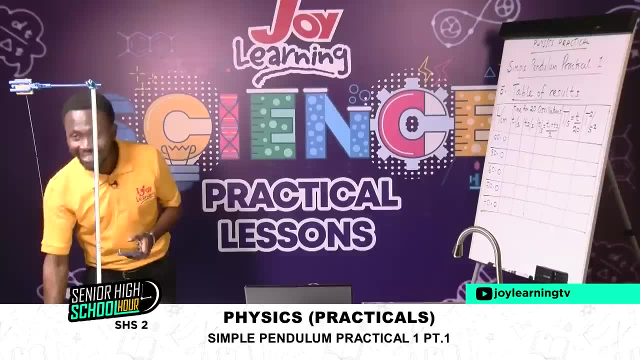 And that is bad. So don't do that, Just displace it through a small angle, Through a small angle. So I'm going to start. So I'm saying: an oscillation is once the bulb is at one end, when you release it, it goes and comes back. 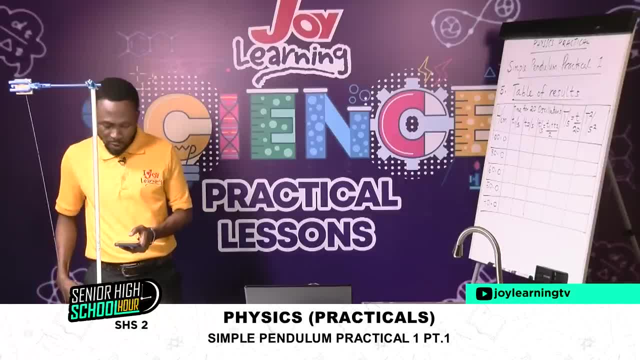 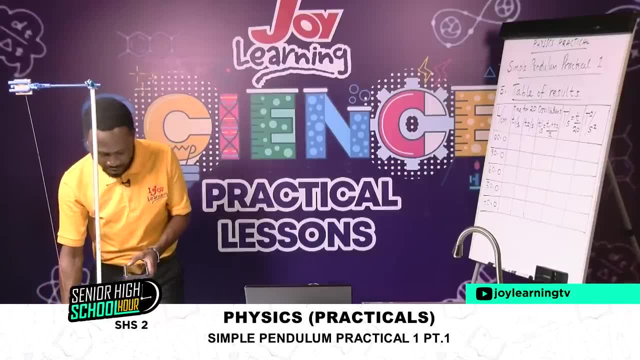 That's one oscillation. So just as you release the bulb, you start the stopwatch at the same time- Very important. So let's try that one. So I have my bulb. this way, I have the stopwatch in hand. 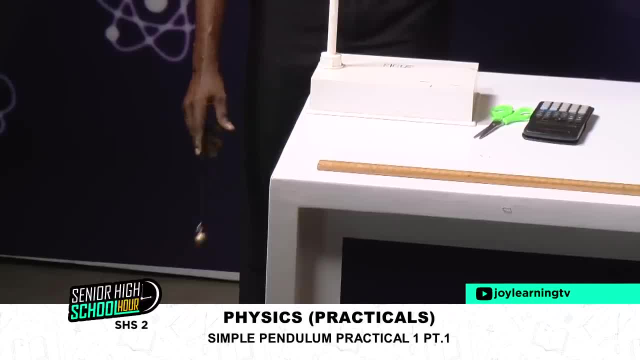 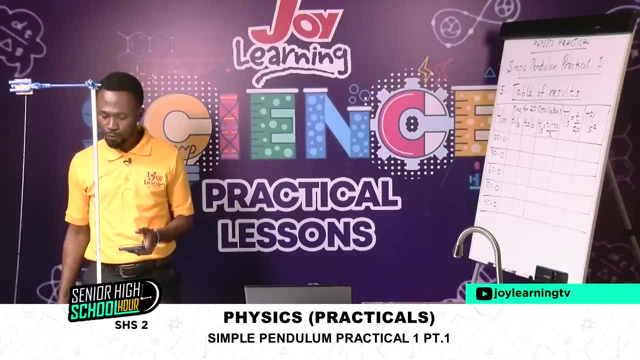 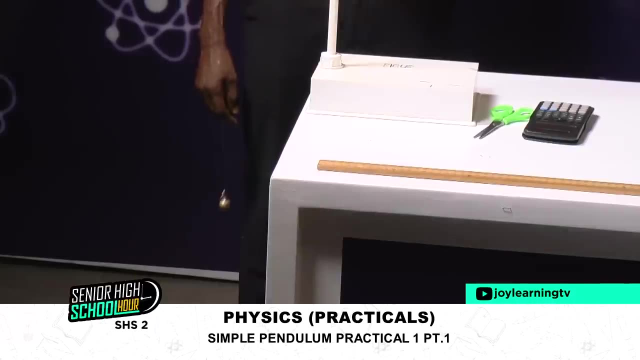 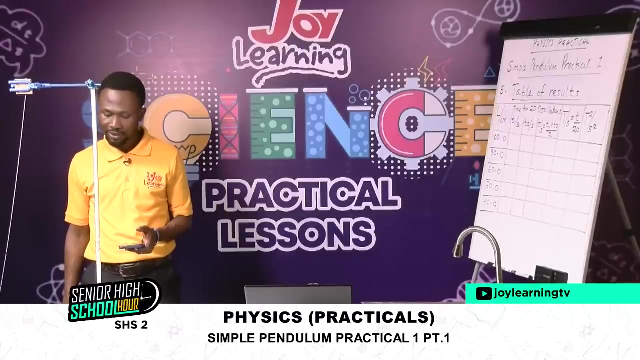 Then, as I release, I start it. So start: 1,, 2,, 3,, 4,, 5,, 6,, 7.. 8,, 9,, 10,, 11,, 12,, 13,, 14,, 15,, 16,, 17,, 18,, 19,, 20.. 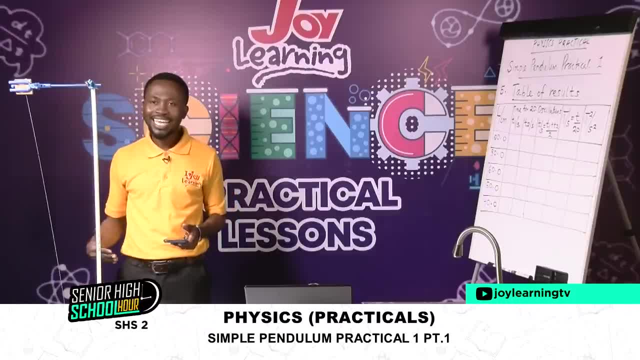 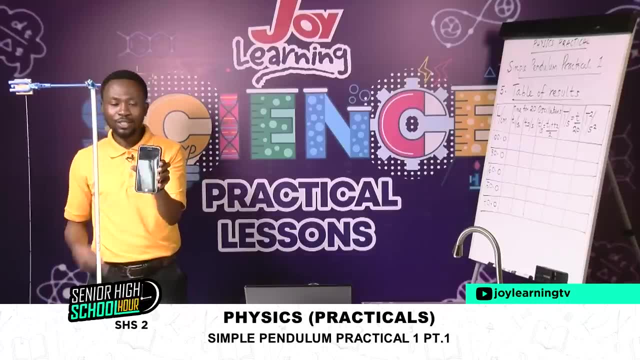 One funny thing is that students, when it's time for 20,, instead of stopping the stopwatch, they'd rather go and stop the bulb. But we need the time rather Now. look at what I have. now I have 004014.. 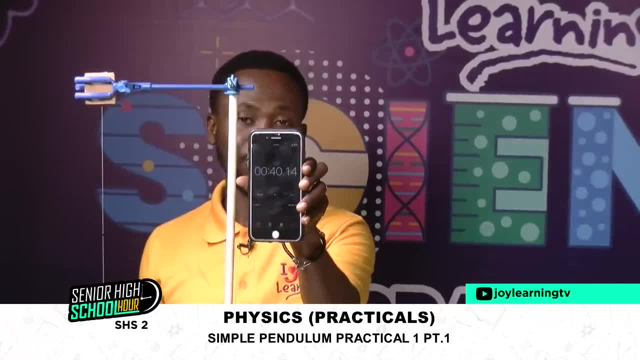 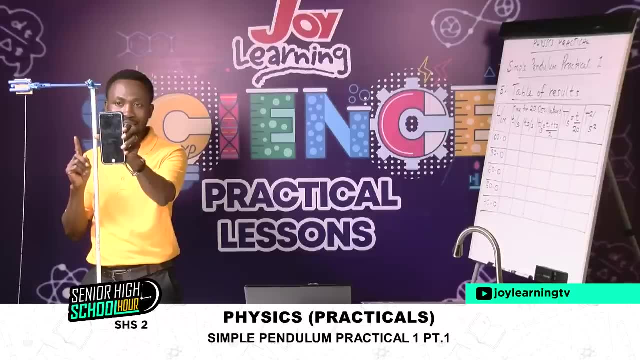 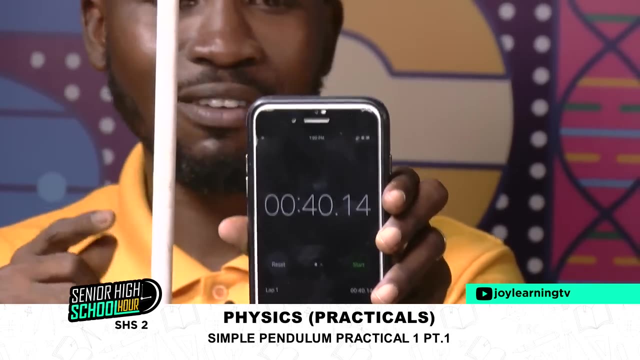 Check it: 004014.. This will be recorded as 40.14 seconds. 40.14 seconds- That's how you record this value. You can see If you had a value here, where you have the 00,, if you have something like 01,. 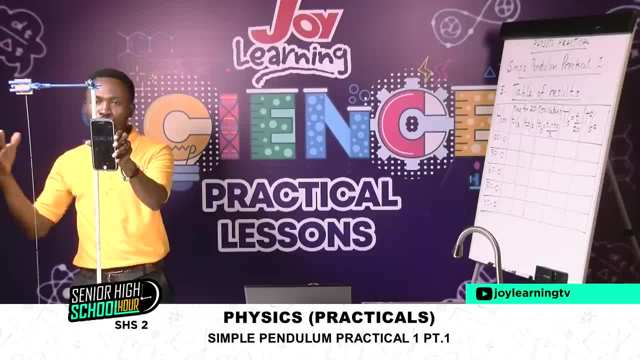 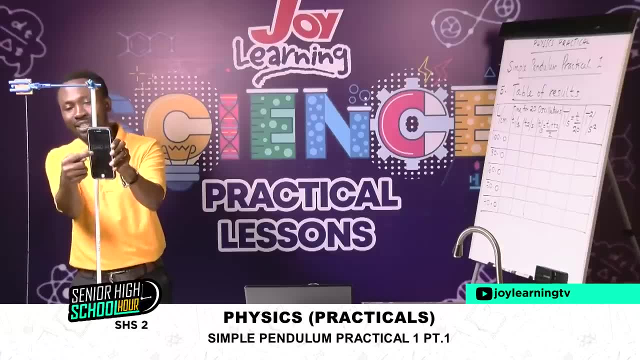 it means you have eaten into one minute, So you change the one minute to seconds. Seconds would have been 60 seconds, So you could have added the 6 seconds to the 40 before the .14.. But here you didn't get into any minutes. 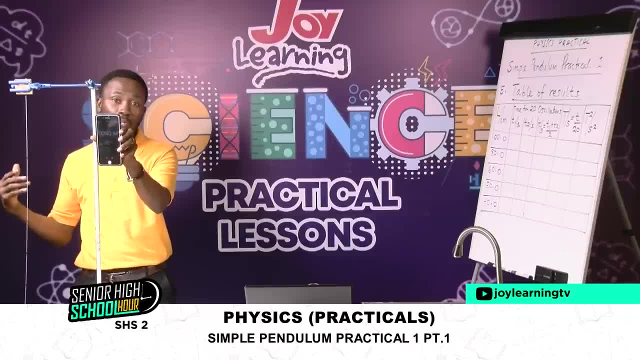 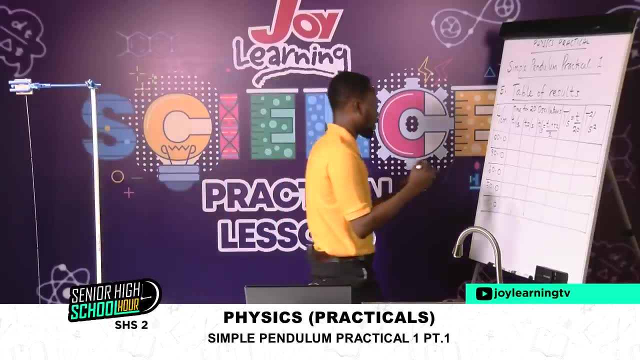 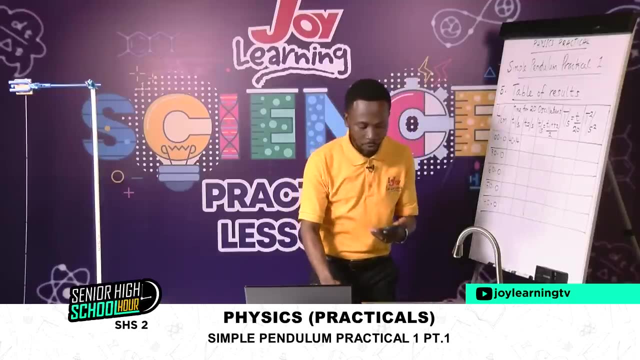 So it is 40.14.. 40.14.. So I go to my table and I record. I put this value there: 40.14.. My first time, 40.14.. Then I'll go to the stopwatch and press reset. 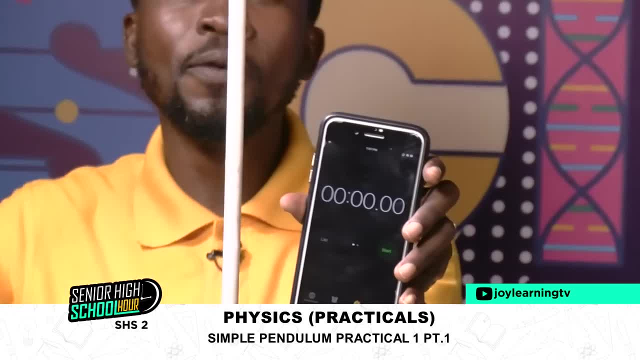 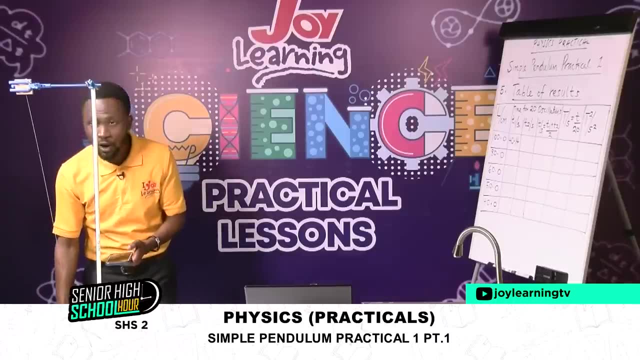 Now I've gone back to 00 again. Then I'll repeat the timing for this length. So we repeat the timing. I display it through a small angle, I release and I press start, So start 1.. 2., 3., 4., 5., 6., 7., 8., 9., 10., 11., 12., 13., 14., 15., 16., 17., 18.. 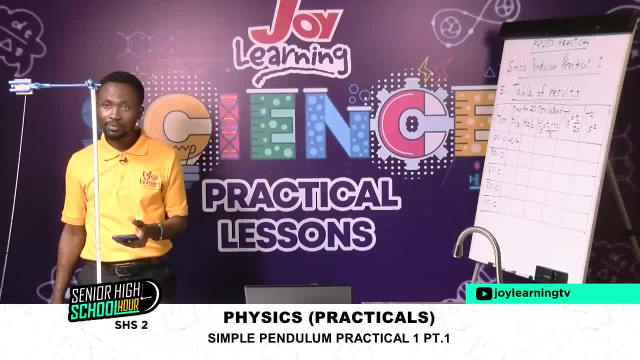 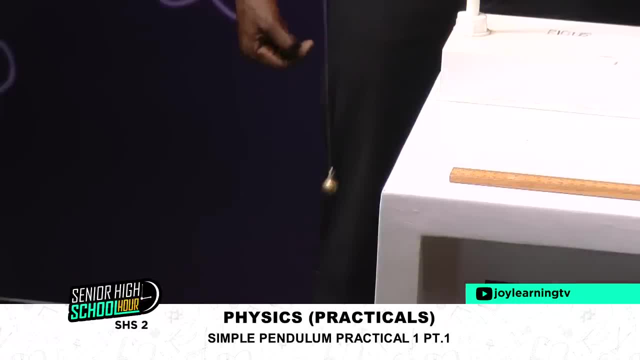 19. 20., 21., 22., 23., 24., 25., 25., 26., 26., 27., 28., 29., 30. 27. 28. 29.. 30., 31., 32., 33., 33., 34., 34., 35., 36., 36., 37., 38., 39., 40., 42., 43., 44.. 44., 45., 46., 46., 47., 48., 49., 49., 50., 51., 52., 53., 53., 54., 55., 56., 57.. 58., 59., 60., 61., 62., 62., 63., 63., 64., 65., 66., 67., 68., 67., 68., 69., 69.. 70., 71., 72., 73., 72., 73., 74., 74., 75., 76., 77., 78., 78., 79., 79., 80., 80.. 81., 81., 82., 82., 83., 84., 85., 86., 87., 86., 87., 88., 88., 89., 90., 90., 90.. 92., 93., 93., 93., 94., 94., 95., 95., 96., 96., 97., 98., 99., 100., 100., 100., 100.. 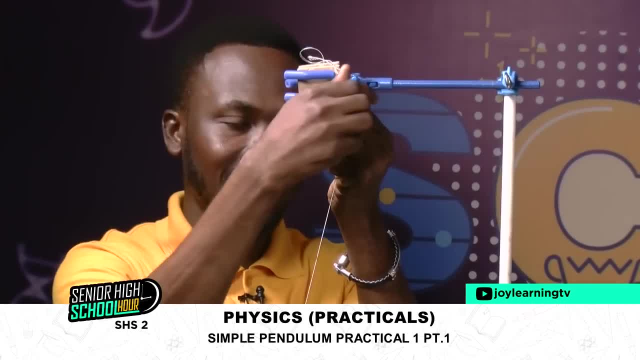 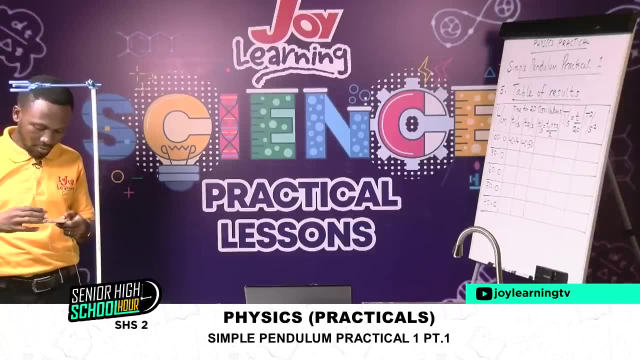 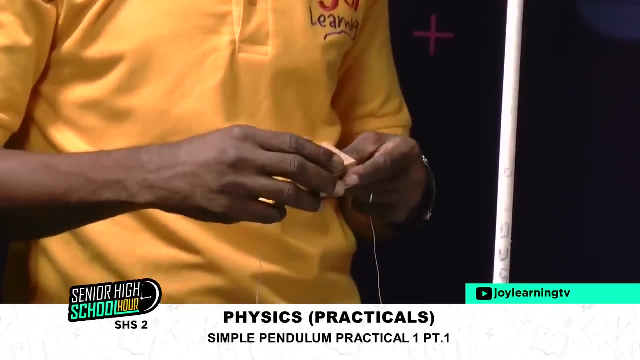 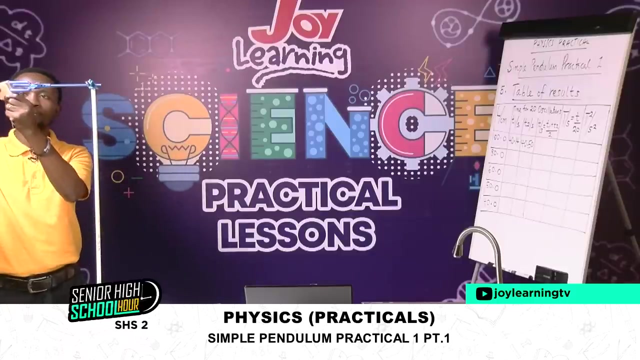 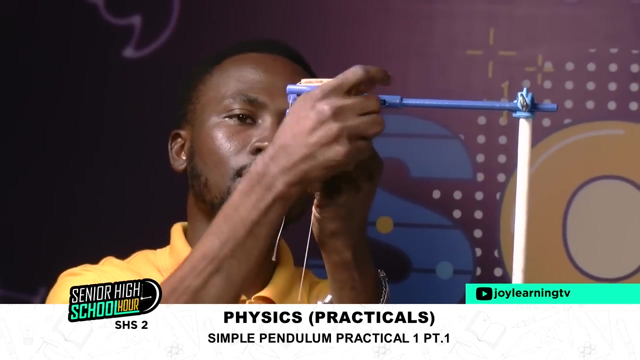 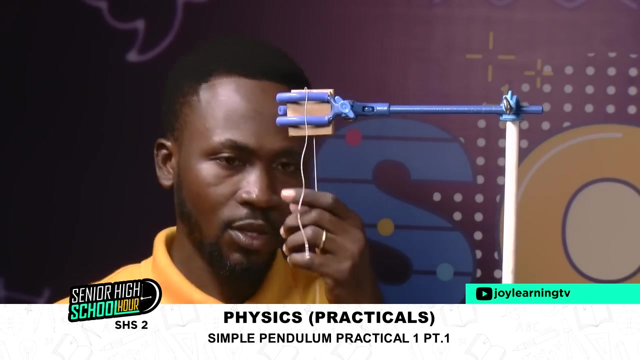 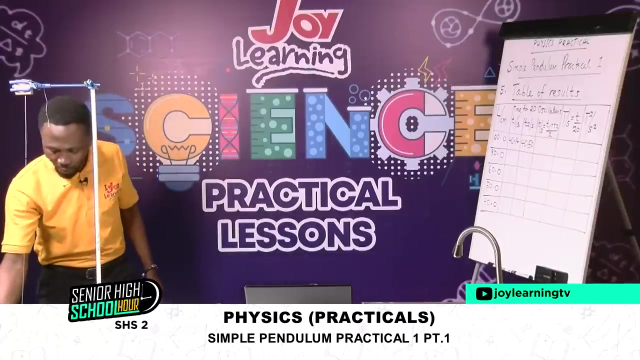 120.. 120., 12., 12., 13., 13., 14., 14., 15., 16., 17.. Then I will suspend again. Good, So this one is giving me from here, from the point of suspension to the middle of the bulb. 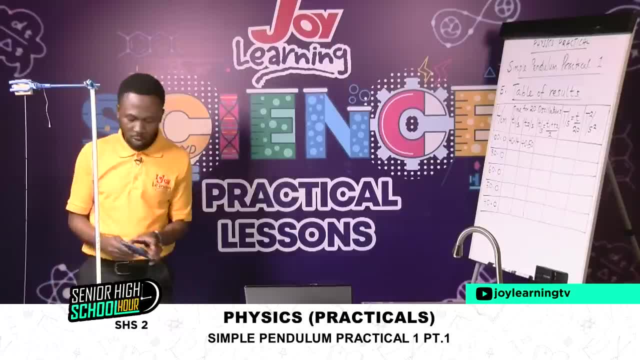 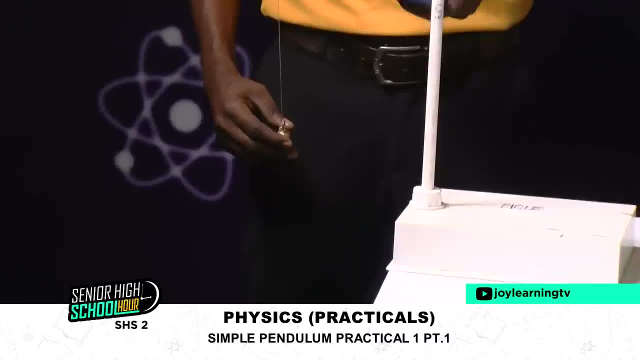 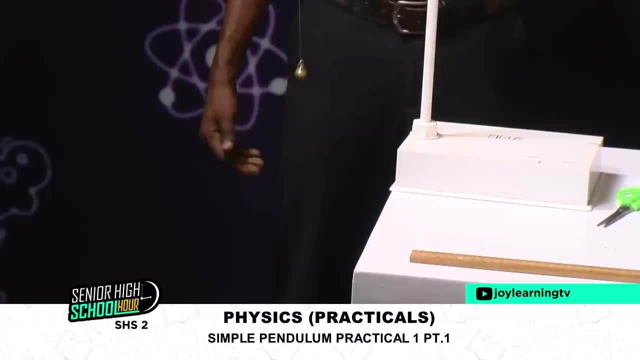 is now 80 centimeters. I take my stopwatch, I displace the bulb through a small angle like that, I release the bulb and then I start at the same time my stopwatch. So let's start. Go One, two, three, four. 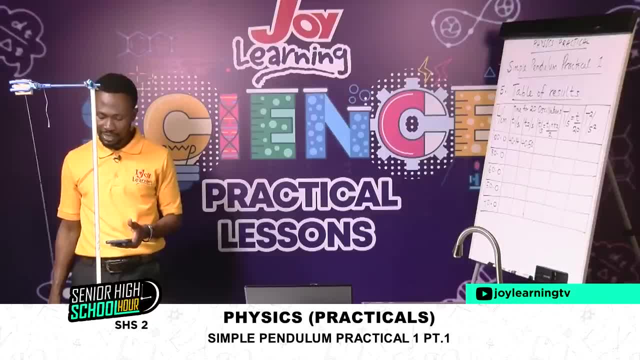 Five, six, seven, eight, nine, 10,, 11,, 12,, 13,, 14,, 15,, 16,, 17,, 18,, 19,, 20.. Then I start again, I stop. 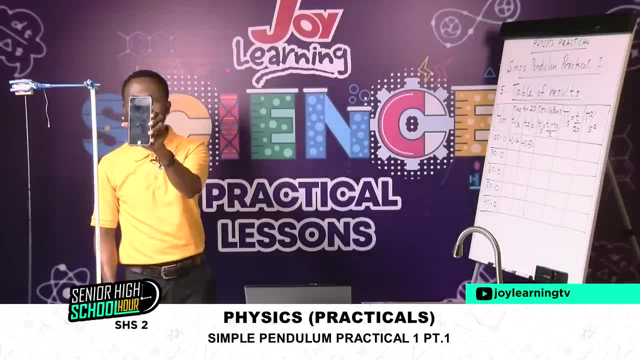 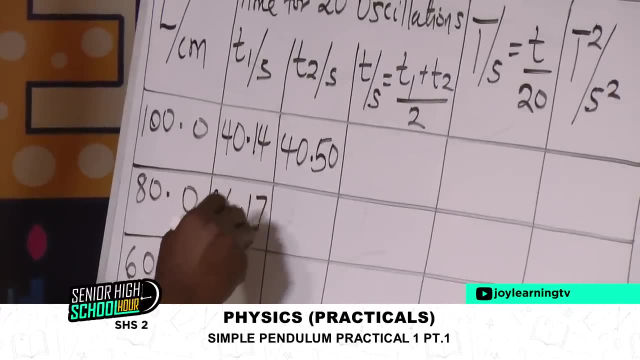 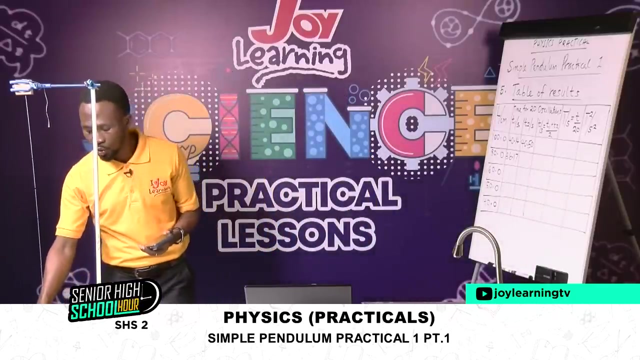 I have 36.17 as my reading 36.17.. So I'm going to record 36.17.. So I have 36.17.. Now we go on. I will restart or reset it, Then go and start for the second timing. 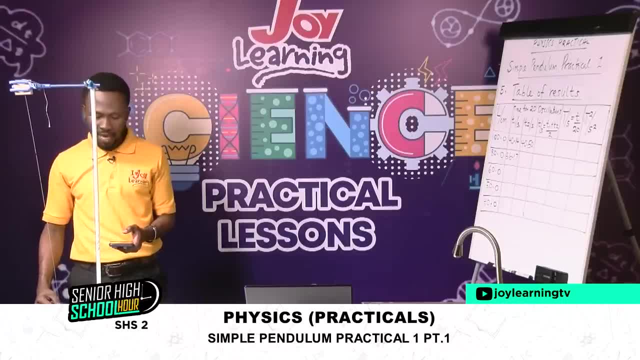 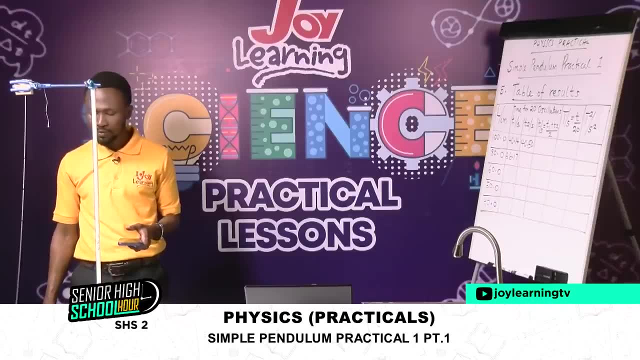 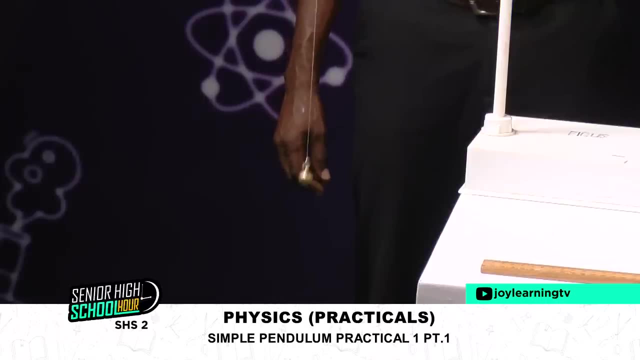 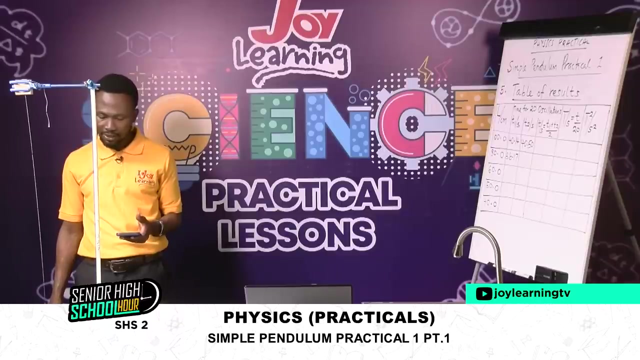 Mind you, I displace it through a small angle As I release it at the same time I start my stopwatch. So let's start. Let's go One, two, three, four, five, six, seven, eight, nine, 10,, 11,, 12,, 13,, 14,, 15,, 16,, 17,, 18,, 19,, 20.. 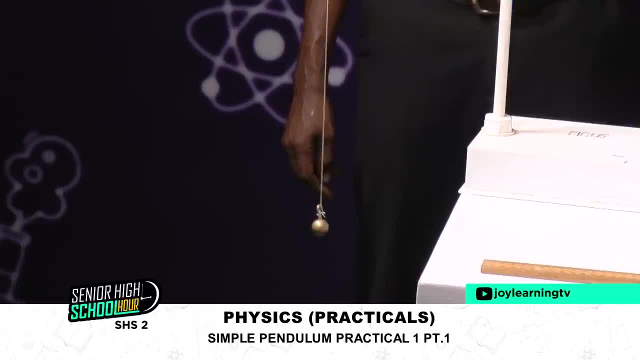 One, two, three, four, five, six, seven, eight, nine, 10,, 11,, 12,, 13,, 14,, 15,, 16,, 17,, 18,, 19,, 20.. 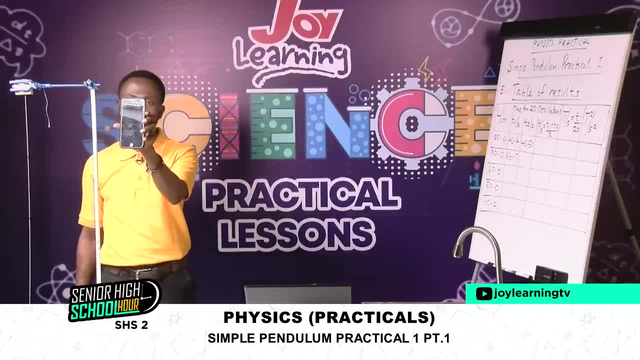 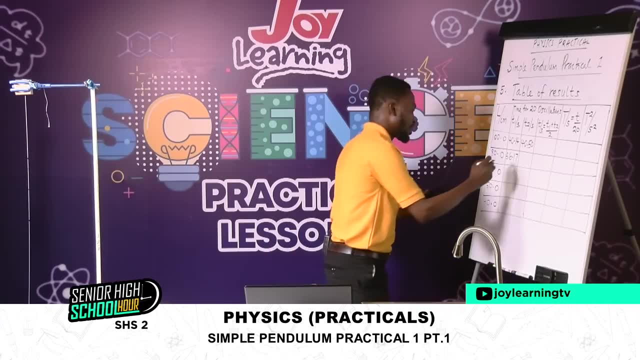 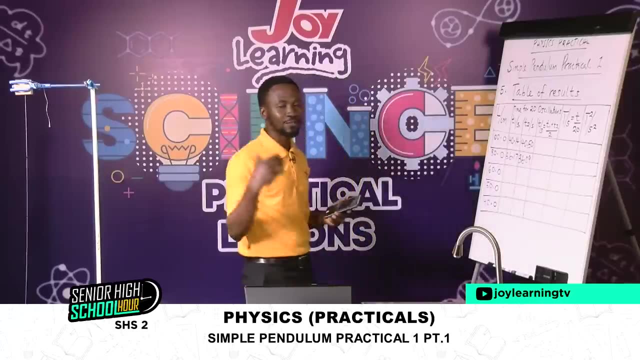 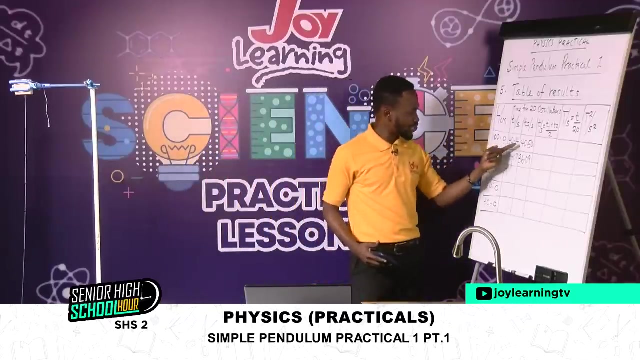 Now I have 36.09.. 36.09.. Very important 36.09.. So I will just put that: So 36.09.. Now You have to take note of what you are doing. When the left was 100, my values were in 40s. 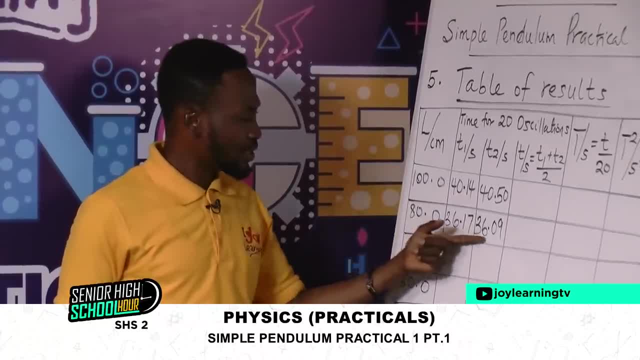 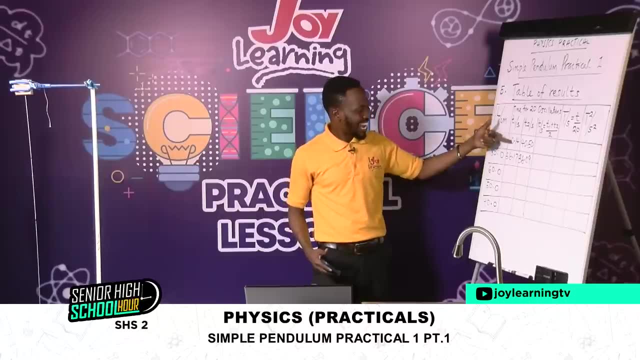 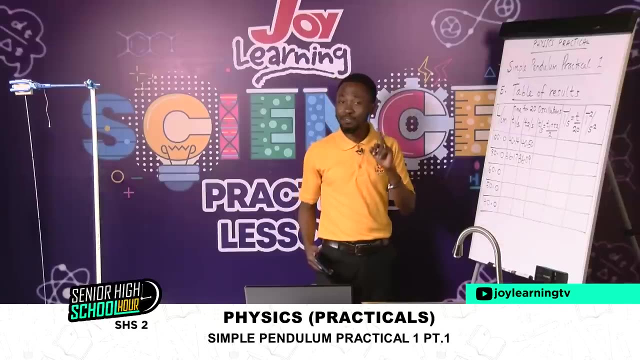 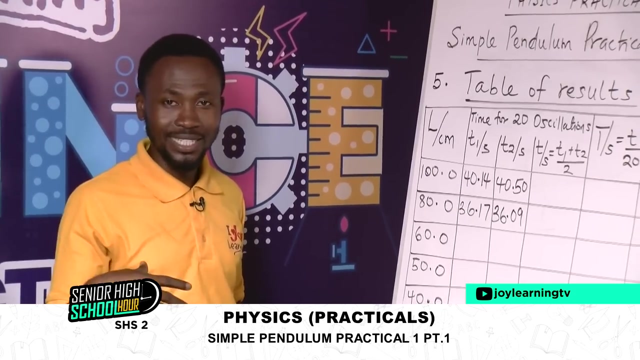 When the left decreased to 80,, my values 36.. Now, As the left is decreasing, the timing are also decreasing. We call that one a trend. In every experiment You must, You must look out for a trend. If you don't find a trend in the experiment, you will score zero for all of the table observation. 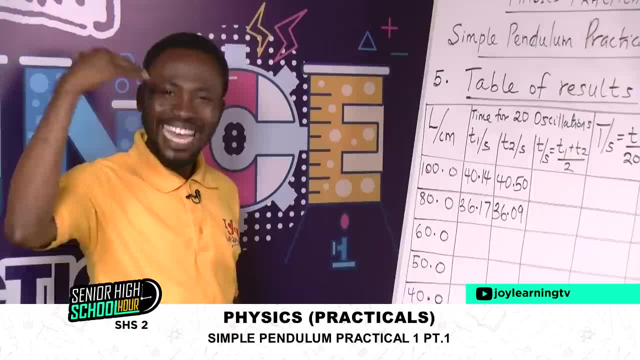 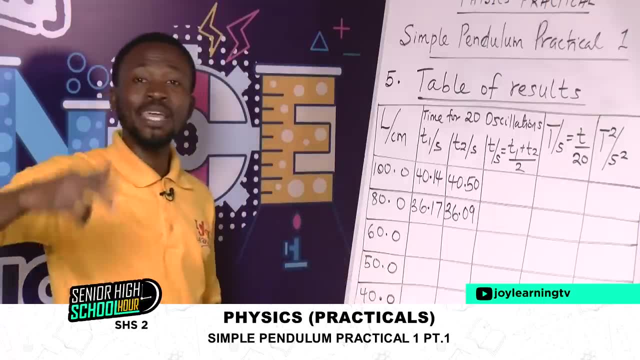 Very important. So it should tell me that in my next readings or timings for 60, I should get something that is below 36.. If I should get something that is more than 36, then there's a problem somewhere and I have to check it. 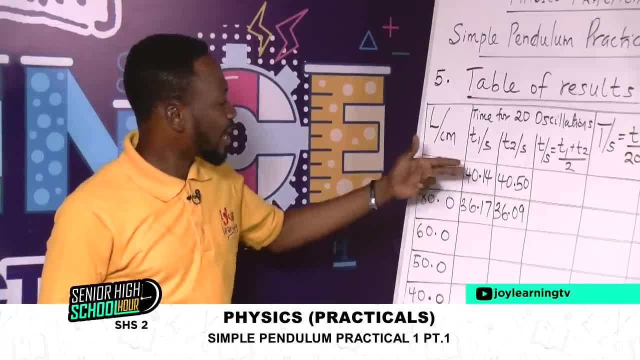 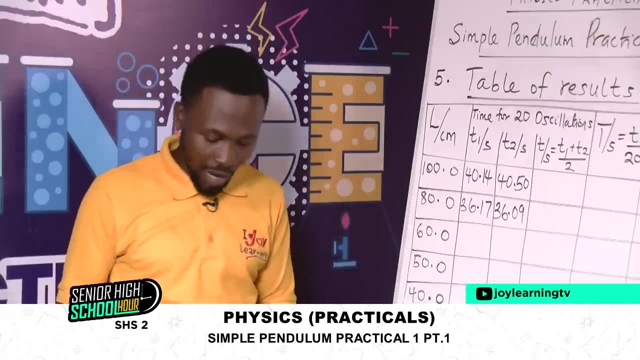 So I have it in mind that The values, The values are decreasing. So my next values should be less than 36.. And it will show. Let's try it out and see. So we are through with the length: 80 centimeters. 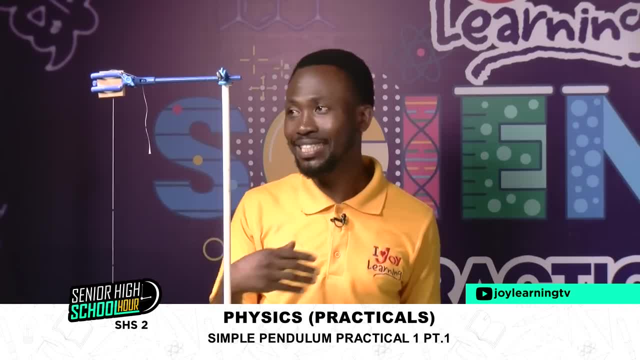 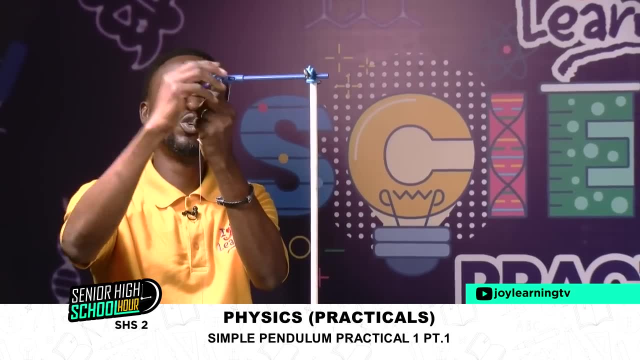 So we go back and we adjust the length to 60. And that is the good thing about it: Once you have the markings, you just have to loosen up a little bit, and then you pull up, You pull up, And then you pull up. 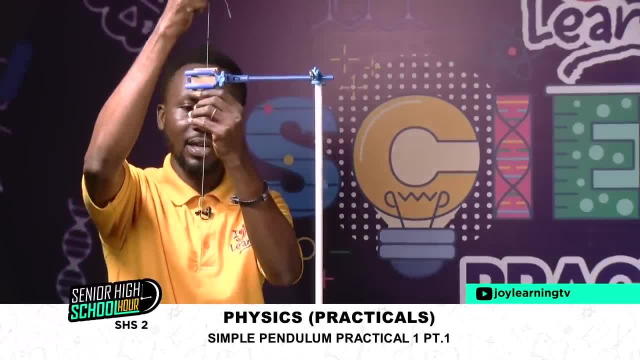 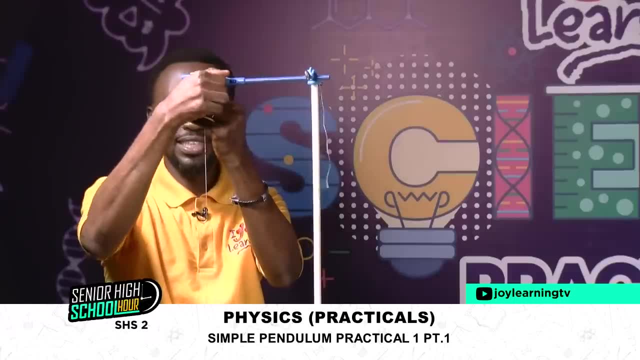 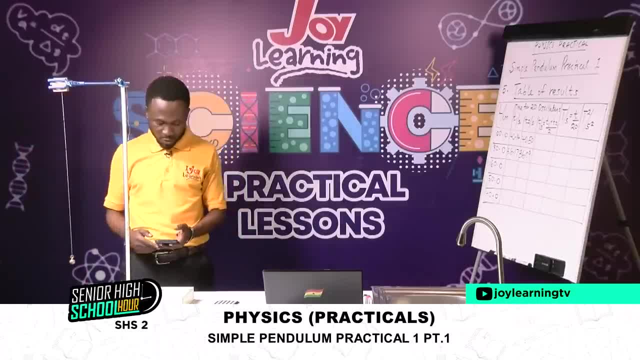 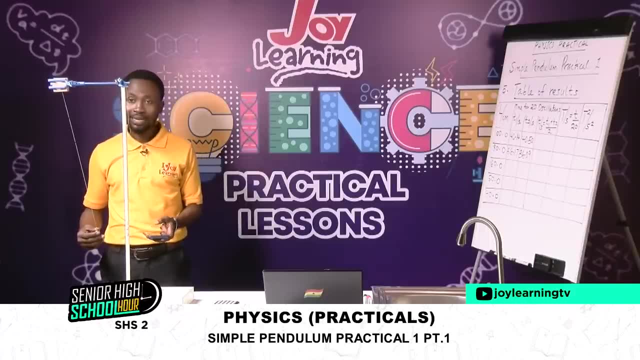 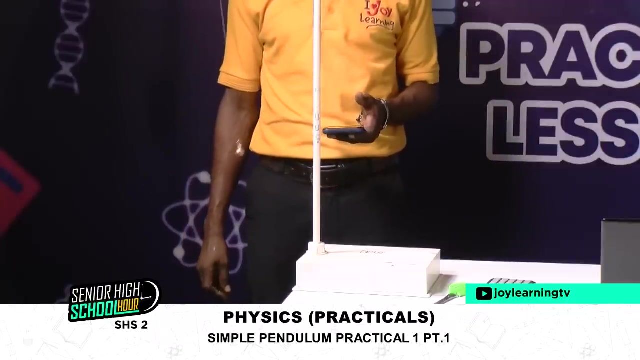 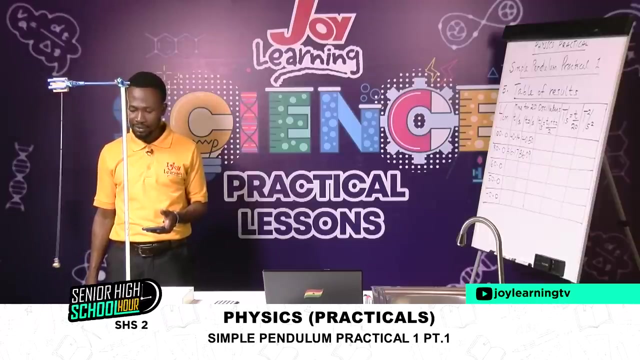 to be 60.. then we also do the oscillation, so i displaced it through a small angle, very important small angle. at the same time i start the stop clock. so let's go one, two, three, four, five, six, seven, eight, nine, ten, eleven, twelve, thirteen, fourteen. 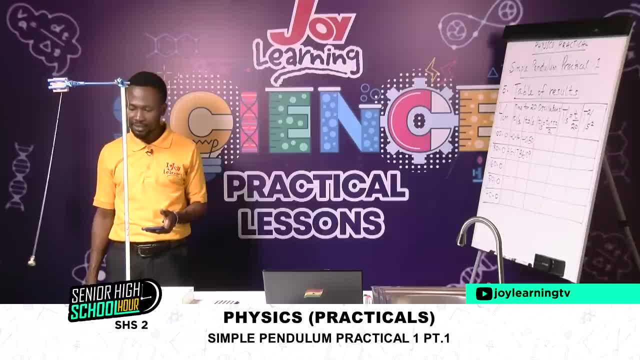 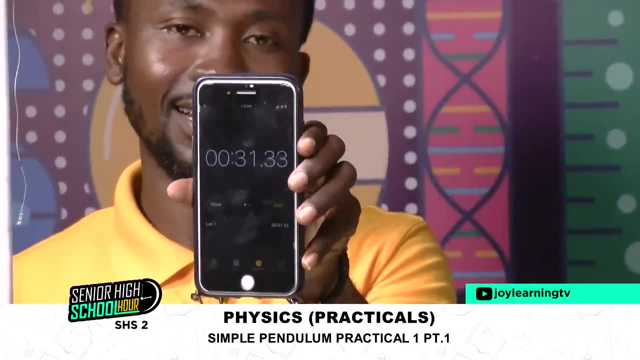 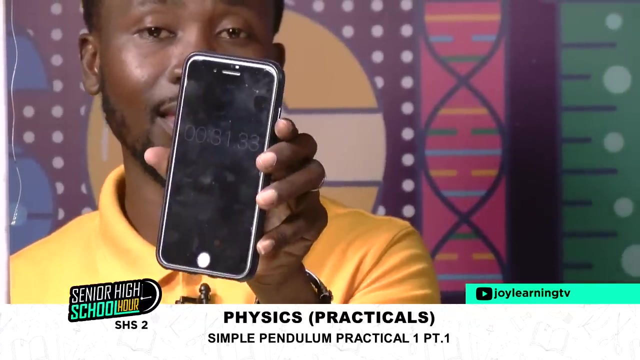 fifteen, sixteen, seventeen, eighteen, nineteen, twenty, and i stopped. so i told you that i expect my next time to be less than 36. other than that, i will not have the kind of trend that i'm supposed to have. so i have 31.33, less than 36, then i should be happy that i'm doing something. 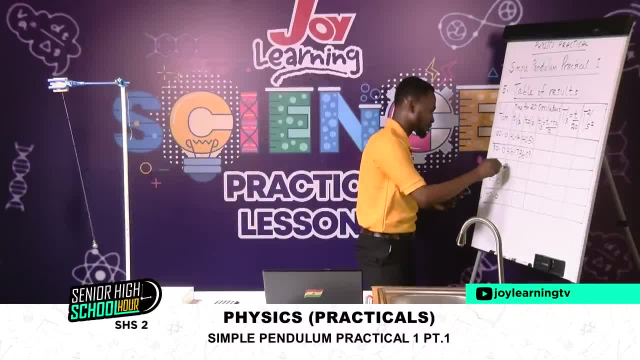 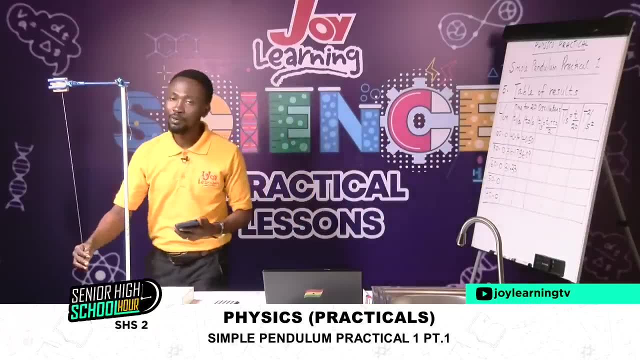 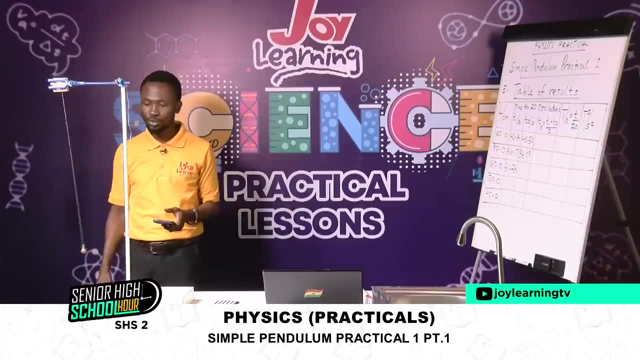 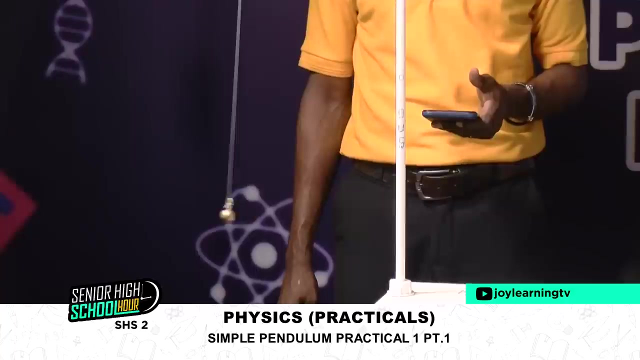 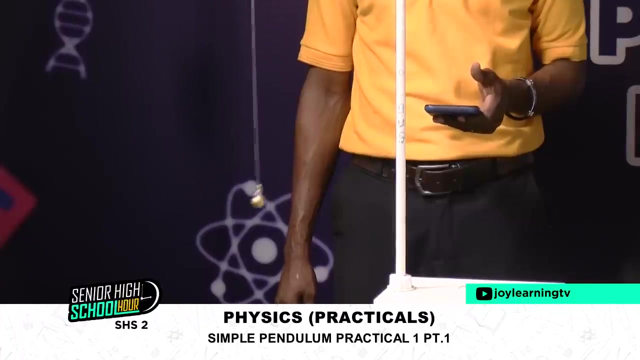 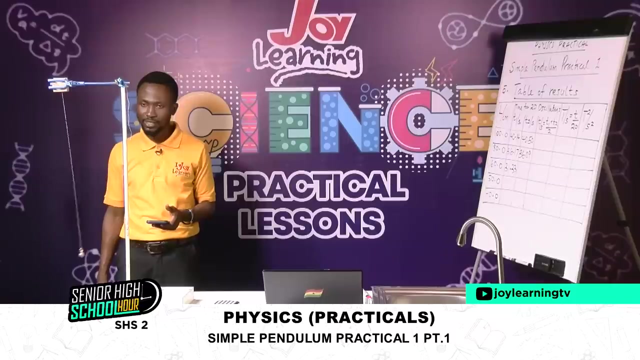 better. so 3-1 and then i'll quickly repeat it. i will reset and repeat for this length: 16.. so start one, two, three, four, five, six, seven, eight, nine, ten, eleven, 11,, 12,, 13,, 14,, 15,, 16,, 17,, 18,, 19,, 20.. 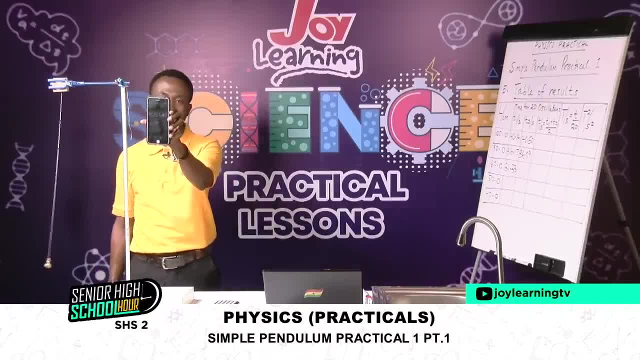 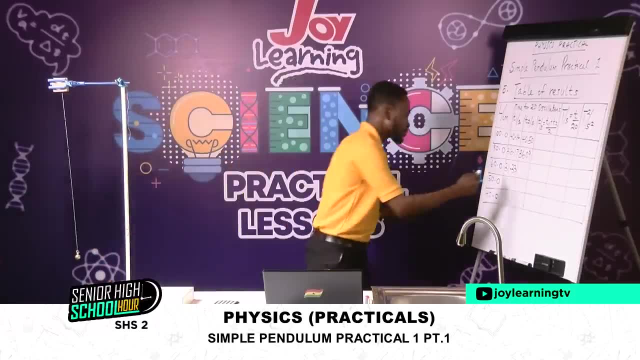 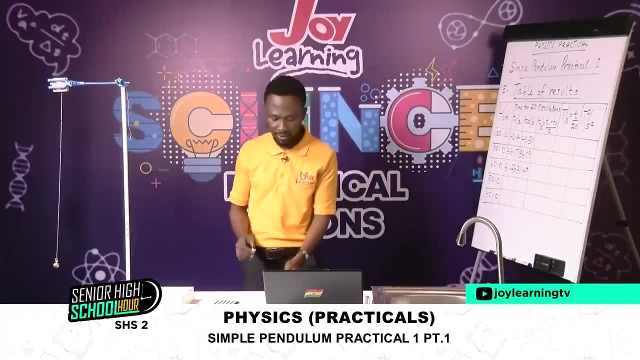 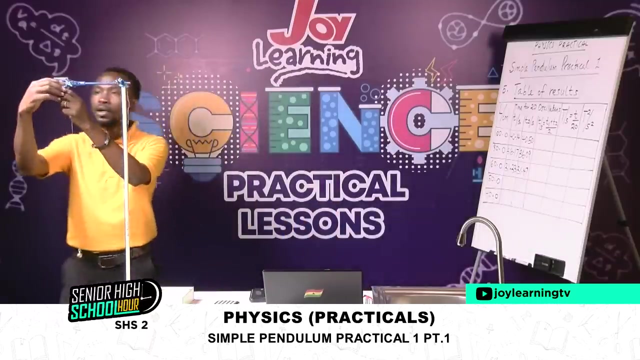 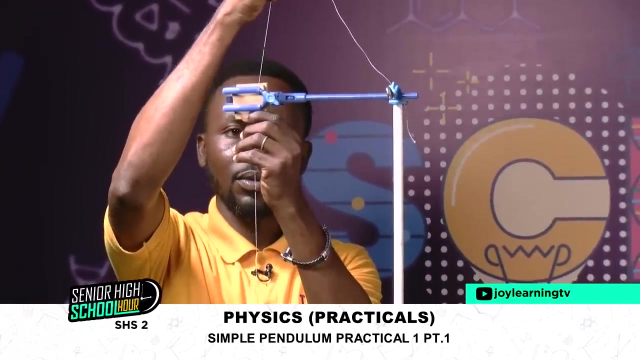 Now I have 31.47.. 31.47 for the second timing. The next length should be 50. So I go and adjust, I loosen a little bit so I can pull, Then I get to 50.. Now tighten it. 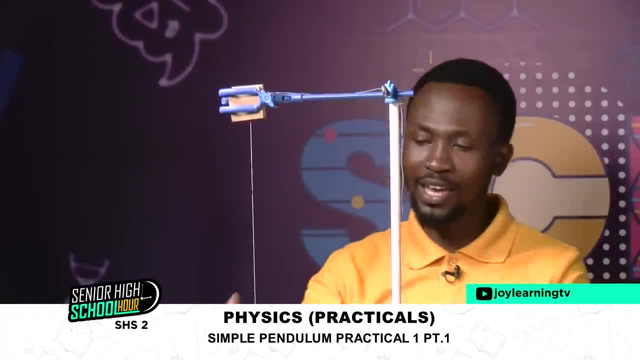 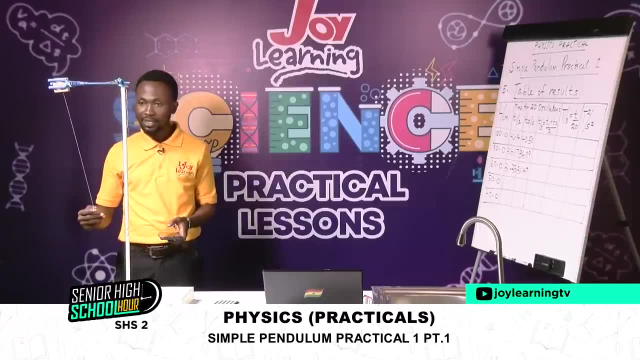 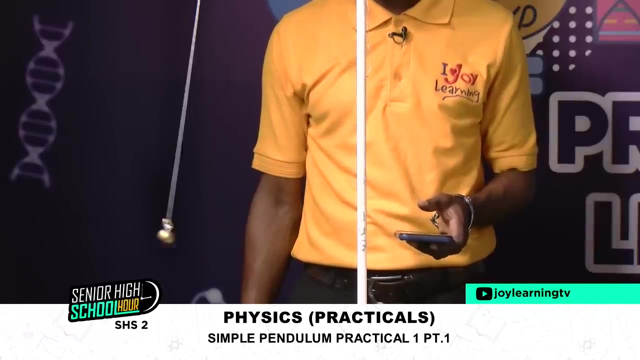 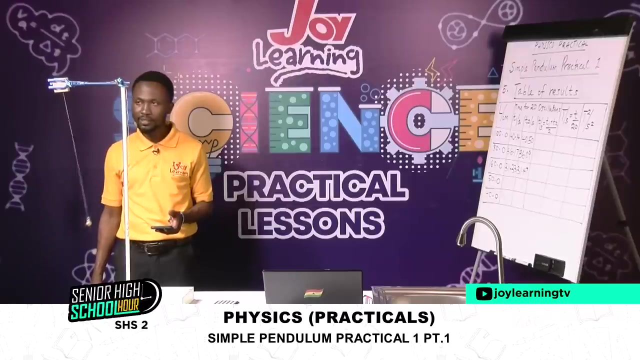 Okay, I make sure that my thread does not interfere with the length What I'm doing Good, So I'll reset, I'll displace And I start simultaneously. So let's go: 1, 2,, 3,, 4,, 5,, 6,, 7,, 8,, 9,, 10,, 11,, 12,, 13,, 14,, 15,, 16,, 17,, 18,, 19, 20.. 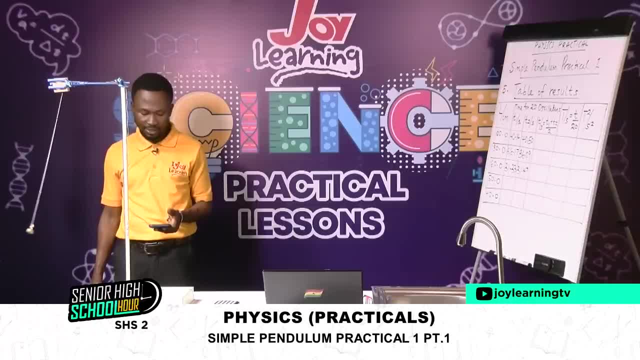 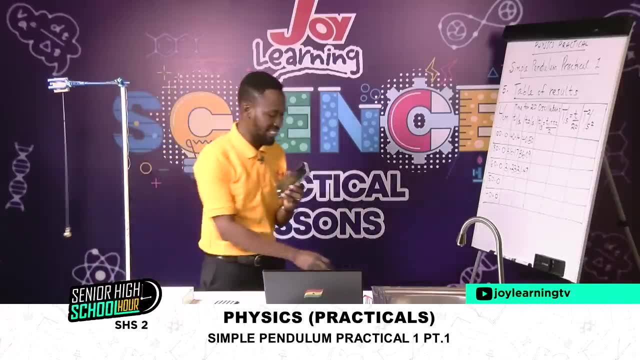 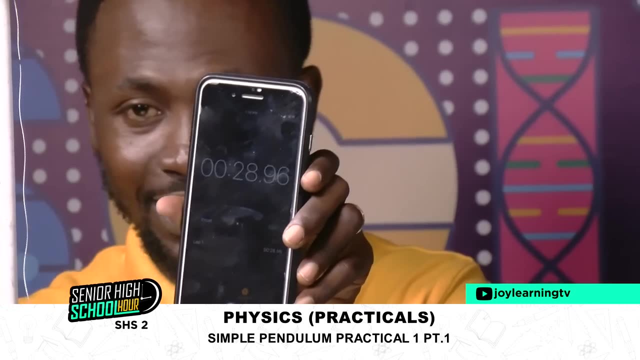 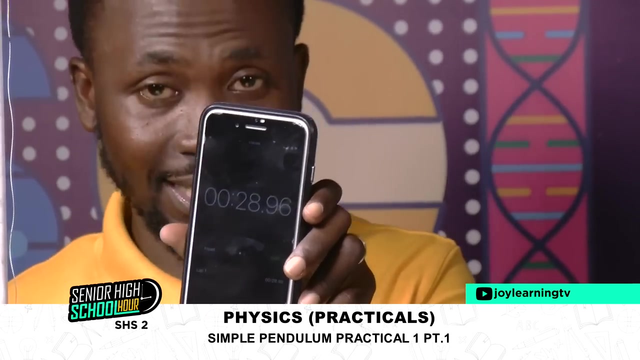 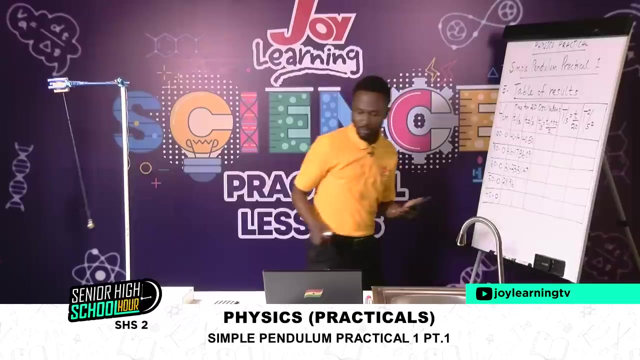 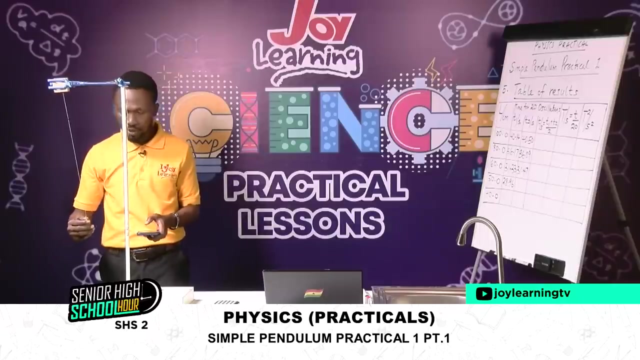 Wow, I have 28.96.. Less than 31.. So we are having a decreasing trend in values, Very important. It doesn't mean that all the time it will be decreasing, No, but there should be a trend. So the most important thing right now is the percentage of the people who will use it. 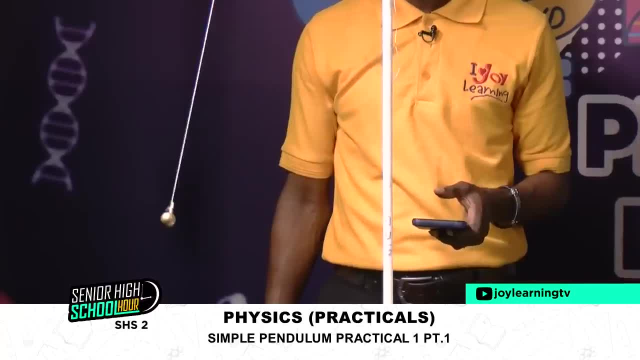 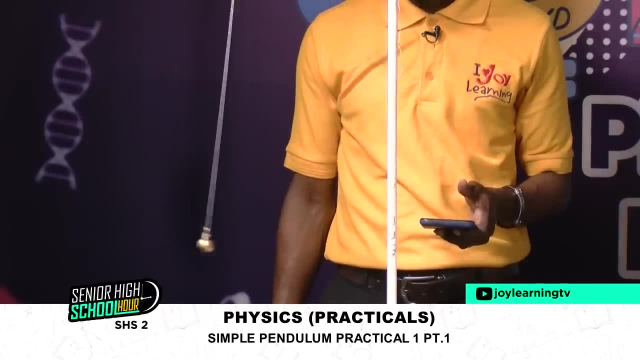 So they will be able to use this method and how to use it. They can't use it now, no, And the second thing, they will be able to use it immediately. So then we get what we've been talking about earlier. So let's go. 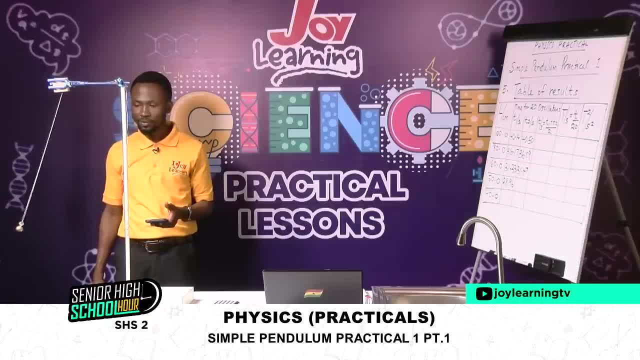 What we're gonna do is: we're gonna do this. It's a quick method. It's a quick method, So we're gonna make sure that you're using it: 14,, 15,, 16,, 17,, 18,, 19,, 20.. 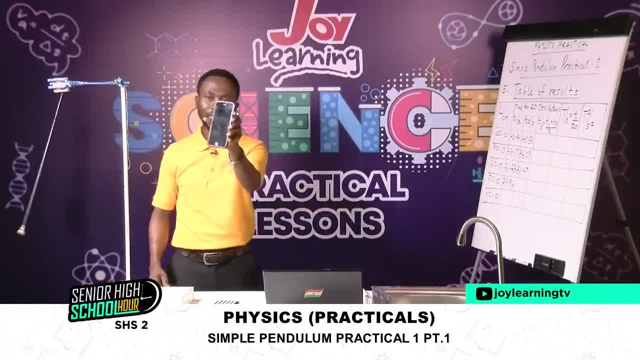 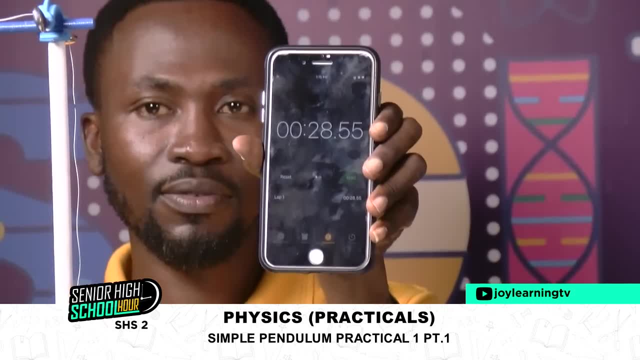 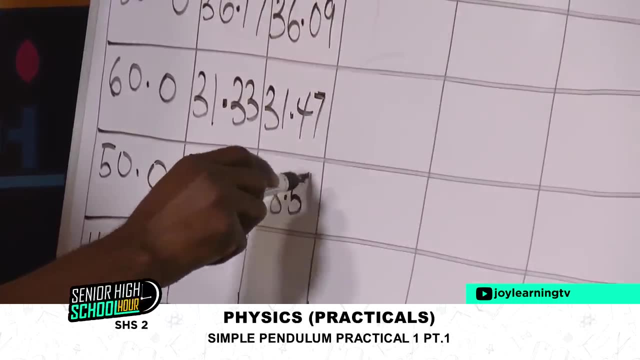 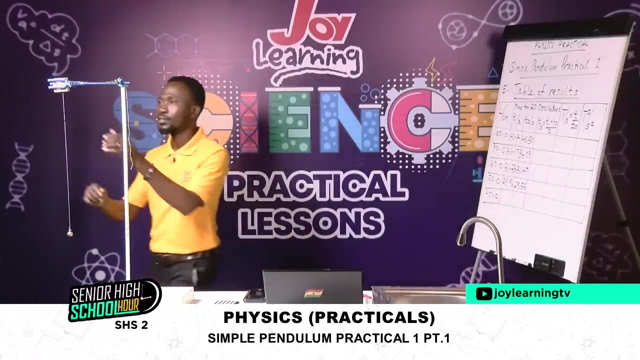 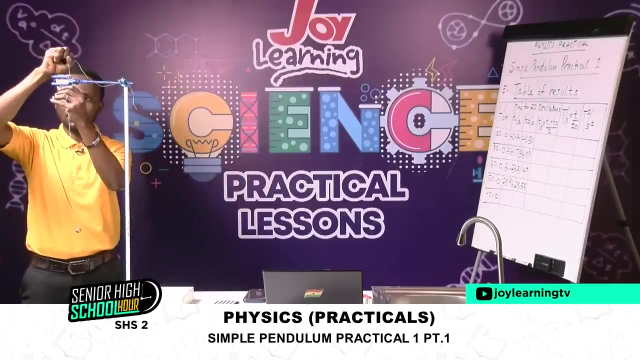 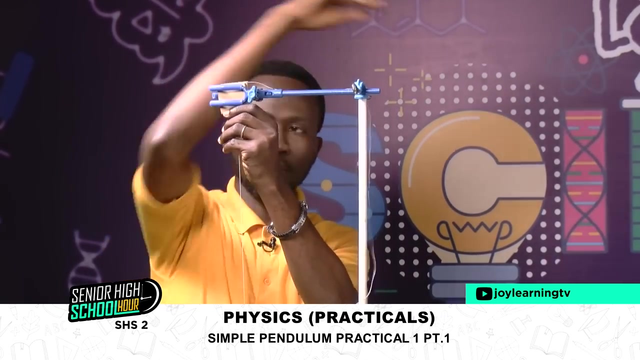 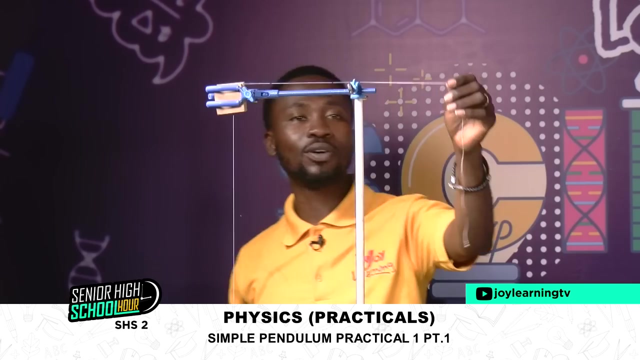 I have 28.55 as my stopwatch reading, 28.55.. Alright, Then our last value, 40. Good, So you see, it's easier and better And faster to get all the readings or the markings on the thread before you suspend it. 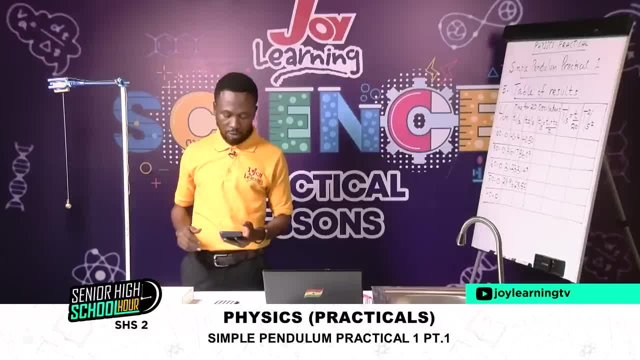 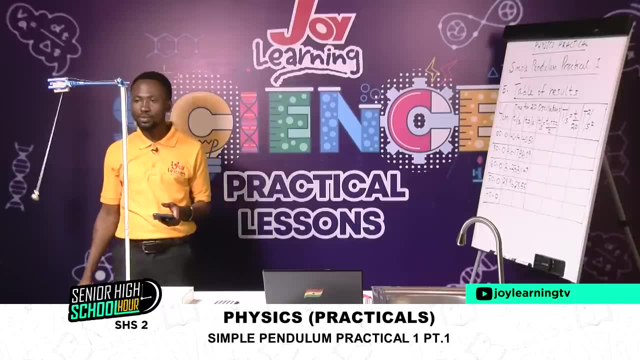 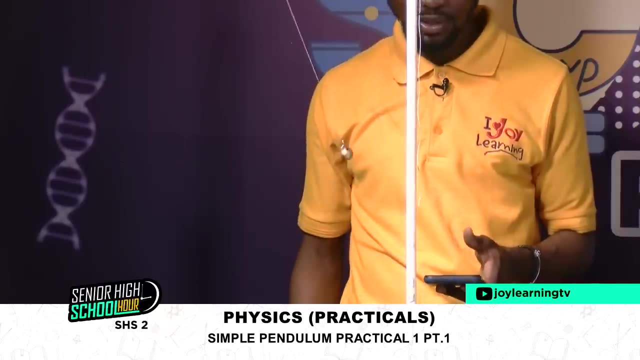 Other than that, you will be wasting so much time, So we reset, I displace it and I start 1,, 2,, 3,, 4,, 5,, 6,, 7,, 8,, 9,, 10,, 11.. 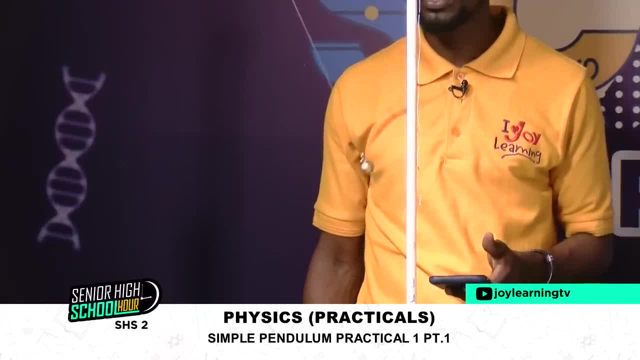 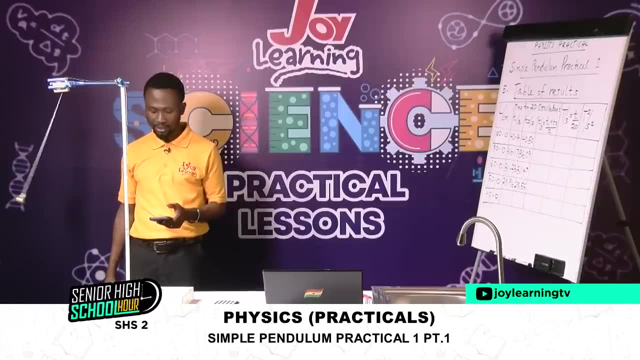 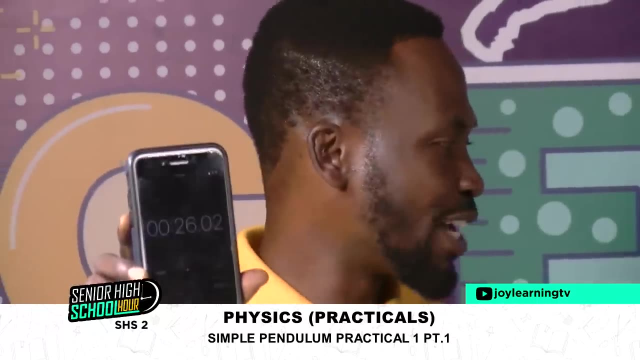 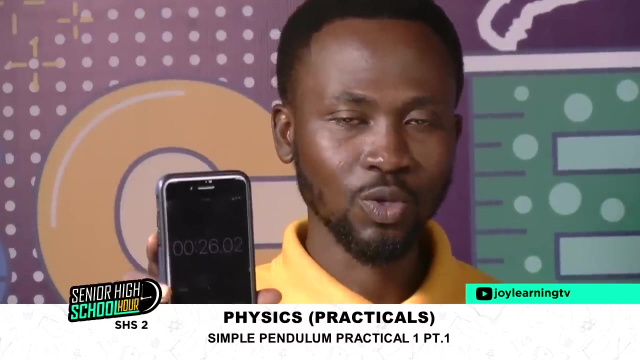 12,, 13,, 14,, 15,, 16,, 17,, 18,, 19, 20.. I have 26.02.. Of course, I know it will be less than 28.. Telling me that my values of my readings are decreasing. 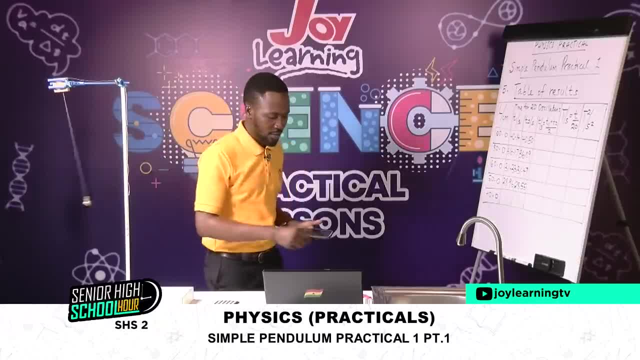 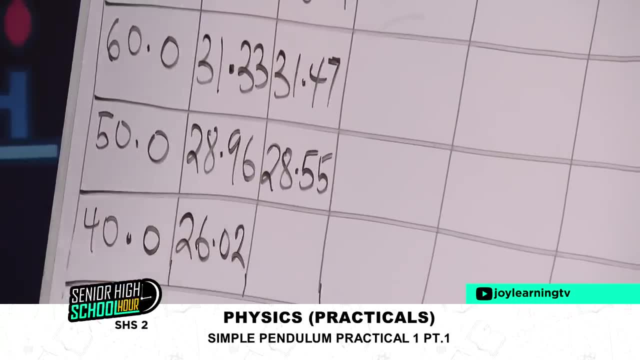 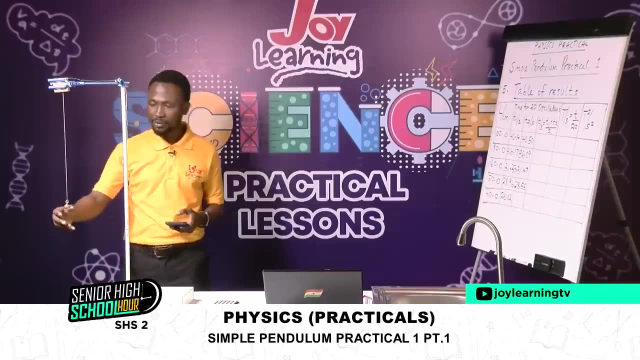 So as we shorten the length, you have less and less time for the oscillation, So 26.02.. Then we try it for the last time: 1,, 2,, 3,, 4,, 5,, 6,, 7,, 8,, 9,, 10,, 11,, 12,, 13,, 14,, 15,, 16,, 17,, 18,, 19,, 20.. 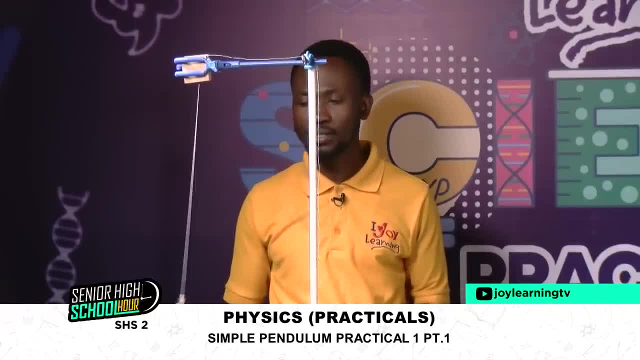 I have 26.02.. I have 26.02.. So 26.02.. I have 26.02.. Then we try it for the last time. Then we try it for the last time: 12,, 13,, 14,, 15,, 16,, 17,, 18,, 19,, 20.. 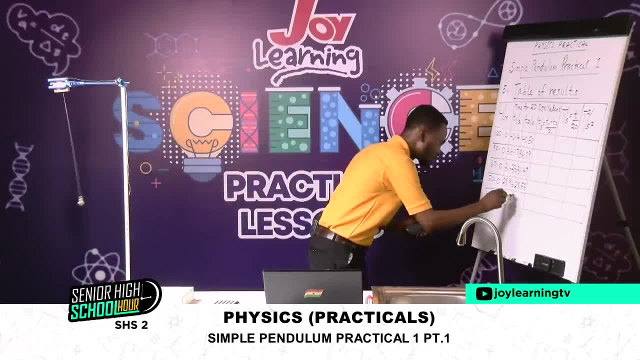 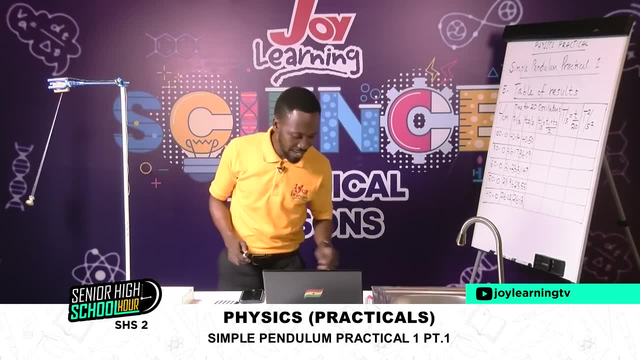 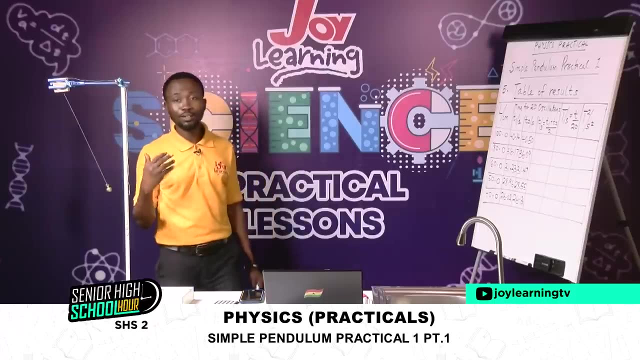 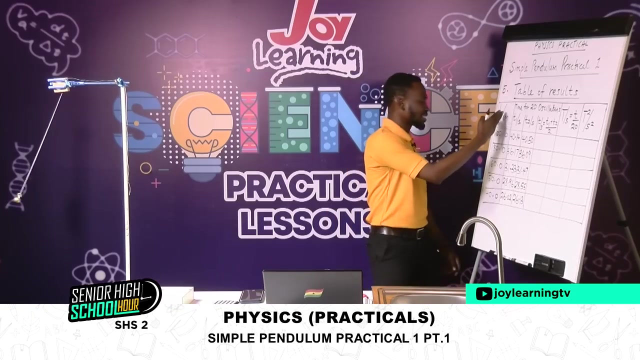 Now I have 26.. 21,, 3.. So whenever the examiner takes your script, he or she is going to look out for a trend in the values. He or she will not look at the lengths, because these were given to you in the question. 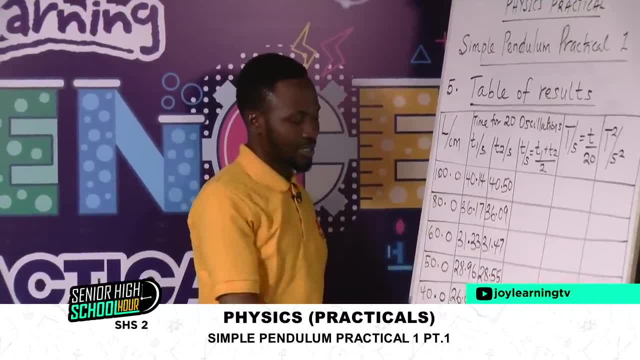 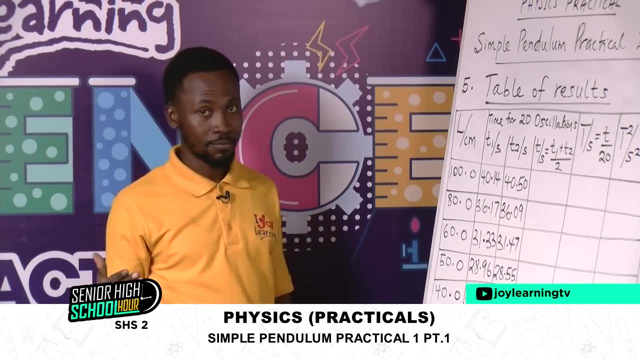 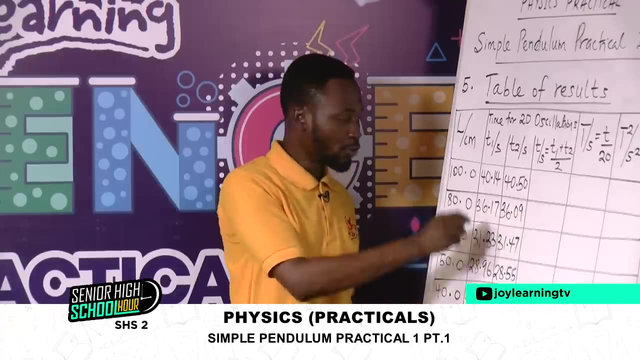 But he or she will look at these Now. the number of decimal places should be the same in each column. So two decimal places for the start and it ends with it Same here. So for each column you should have the same number of decimal places.